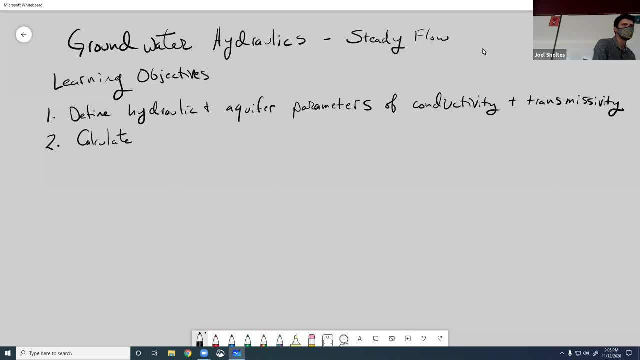 calculate hydraulic conductivity- these parameters- and transmissivity, um, oh, okay. so calculate these parameters or we'll calculate groundwater flow rates using these parameters. so we'll calculate flow rates using these parameters and darcy's equation, also the deploy. i'm not going to pronounce this depute, depute equation. 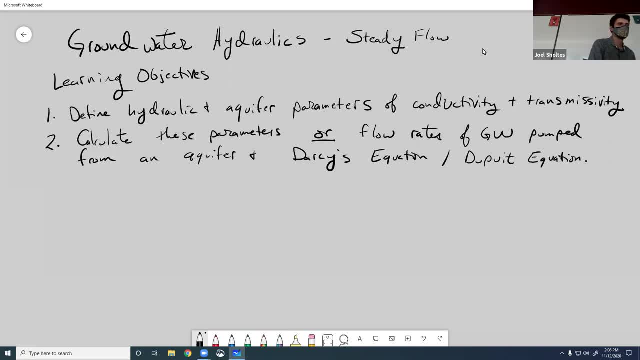 i think that might be french val. can you help us out? okay, did we, did we? thank you, and we're going to apply- not even close to apply- these equations to characterize what's known as the cone of depression around a pumped well, so where we're withdrawing water from a well. 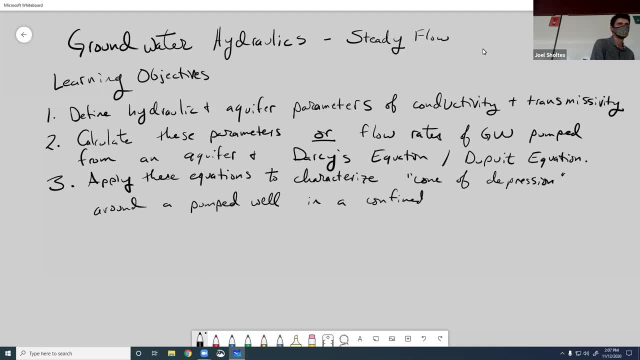 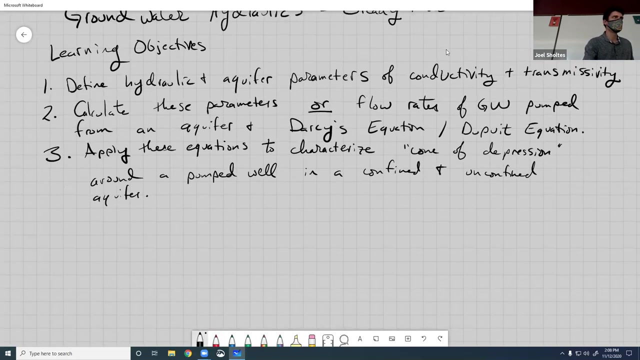 and a confined and unconfined aquifer, all right. so hydraulics again is referring to the kind of physics of flow, flow rates and how we calculate that. all right, and that's um, that's pretty much everybody's goal, especially with many of the yea us, California. 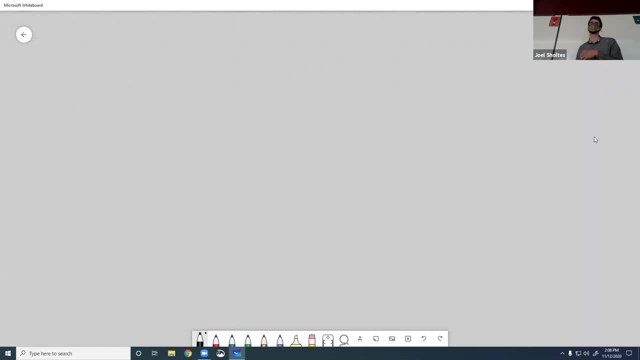 to think about biscuits and aerosols, but let me remind you, think about the procedure. endos paralyzes the solid byoshaid defence, pelo cras. That's what our lab, nice neighborhood with these and it. that was the idea. how do you say this? right? I don't know what you call it. would you consider to look at how much? 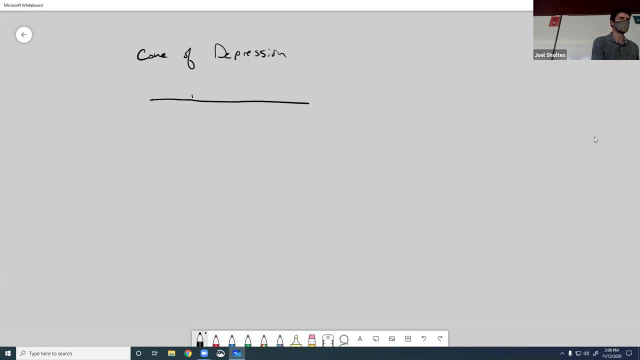 We saw some a cartoon of that. So if this is the ground surface and here's our water table, you put a well in there that penetrates through the water table and you start pumping out at a certain flow rate. The cone of depression is what happens around the well. 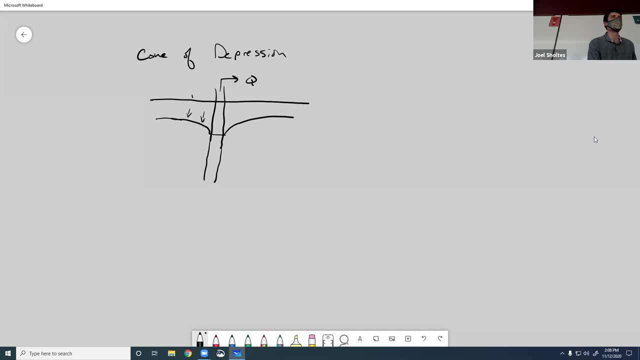 And so you would call it a lens, a groundwater lens. and that can happen and we saw when we had a river during a flood. we maybe the groundwater during base flow looks something like this, but then a flood event comes and all of a sudden water is over the floodplain. 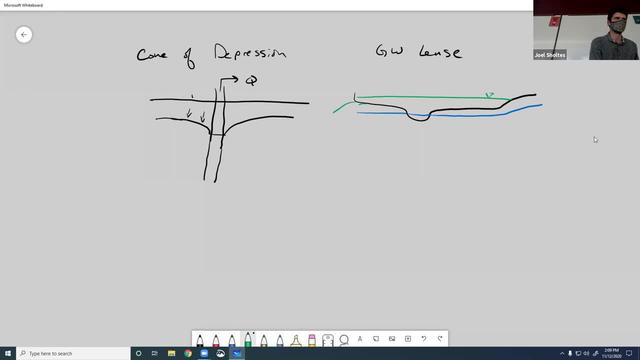 And then we start to get the water table rises and kind of, you know, fills in this way right, And that would be kind of the opposite of a cone of depression. So that can happen during floods. that can certainly happen from a reservoir. 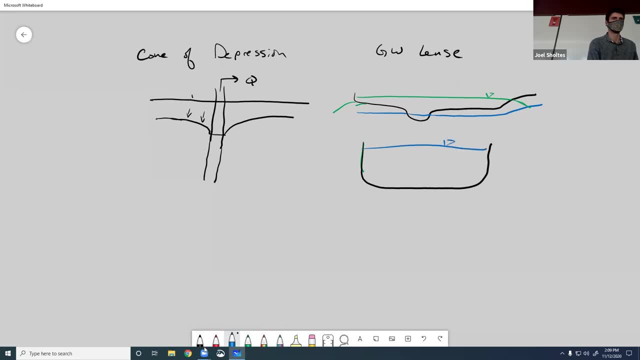 where you've got a big water level and it's a reservoir that's perched, and then you know, the creek used to be down here, but now you've got basically a water table that looks maybe something like that, or it might look something like that: 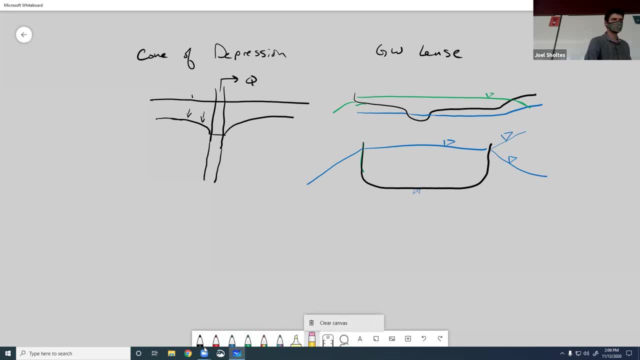 So we should be able to get that up there, And if it's not, I don't know. But that's about it, Okay, so let's get to this next one right here. So we're gonna go back to our water table. 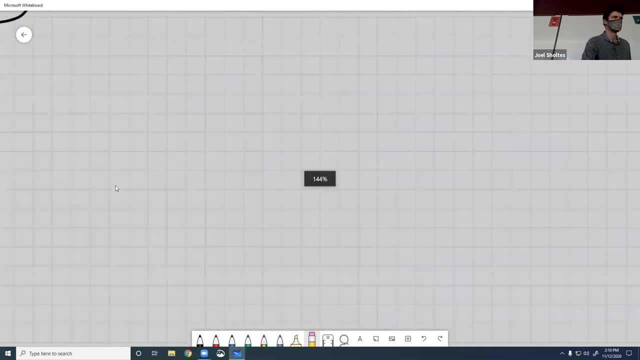 So again, it's the same method as we did on the big water table, but we're gonna go back to the water table and go ahead and try to find the first water thing that we're looking at. So we're gonna go back to our water table here. 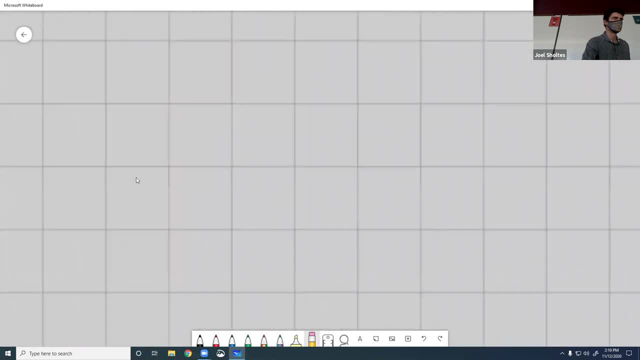 and we're just going to go back to the water table and we're going to go ahead and click on this thing and we're gonna go ahead and down here and then we're gonna go back to our water table. So that is the water table, on our water table. 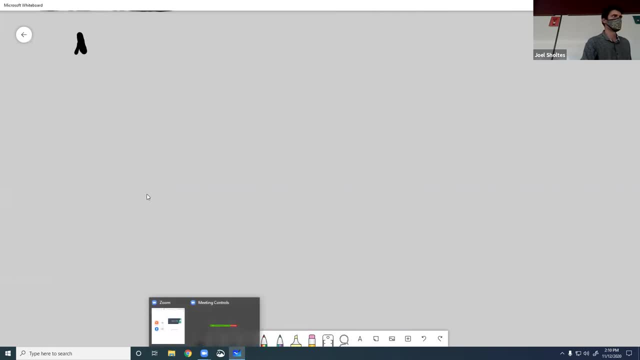 So the water table and we have a lot of different ways to determine Aquifer properties. the first one we talked about was permeability, and that was lower case. k is equal to some coefficient times the diameter squared and it has units of length squared- The diameter. does anyone remember what diameter we're talking about? 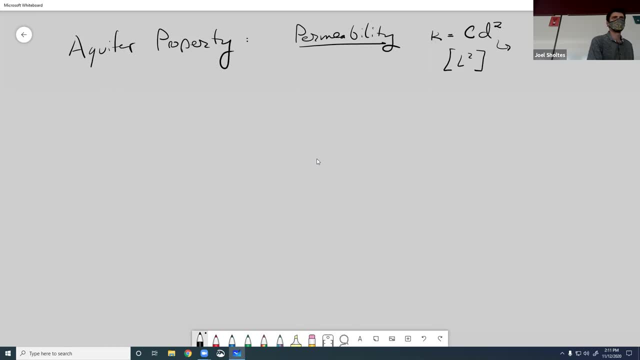 here: Grain size. This would be the mean grain size. Sometimes it might be the median, but we'll talk about that. So if this is a soil sample, sandy, gravel, cobbly loamy, you can measure this directly. This gets a little funky. C is a shape factor. 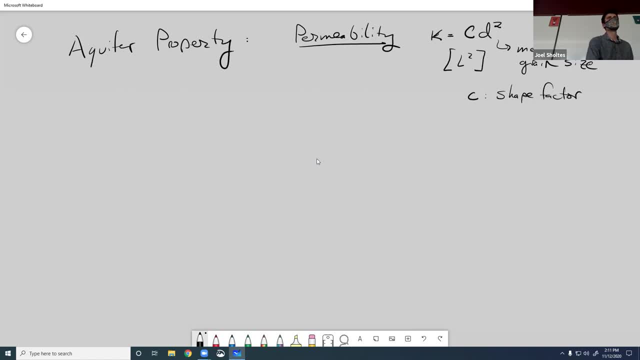 Right, Yeah, D50 is a median grain size. That's often what's used in soil. This says mean People might use those interchangeably, but they're not always the same. And then we learned about conductivity, which was not only a property of the soil or the aquifer itself, but it 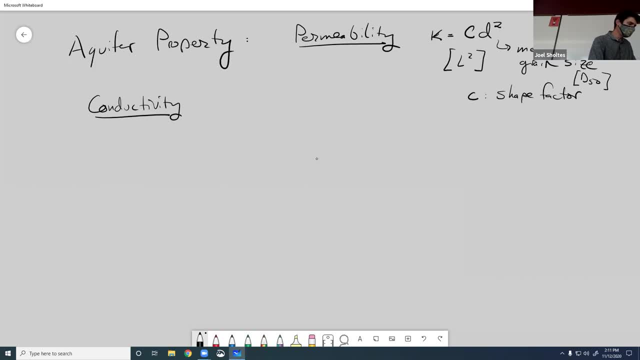 was a property of the fluid as well, And that's big K. This is little k, And big K is equal to little k times the specific weight of water divided by the dynamic of viscosity. And then we also talked about porosity, eta, which is hurricane eta flying over. 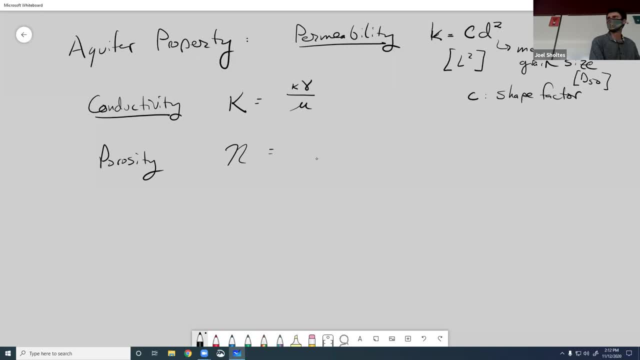 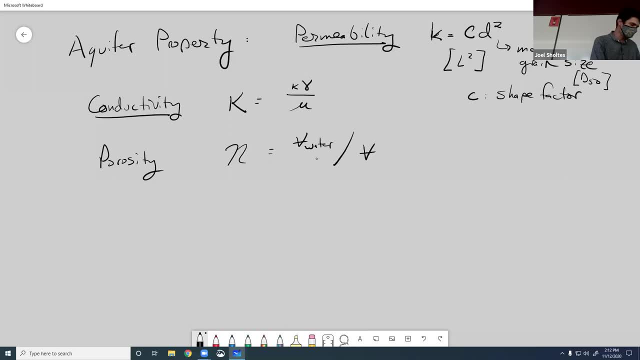 know if it's a tropical storm or Attaway, but anyways, that's. that's the volume of water over the volume of your. I'll just say total of your sample: No evacuation. I don't think it's that big of a storm. My mom hasn't been texting me or anything, so it's okay. 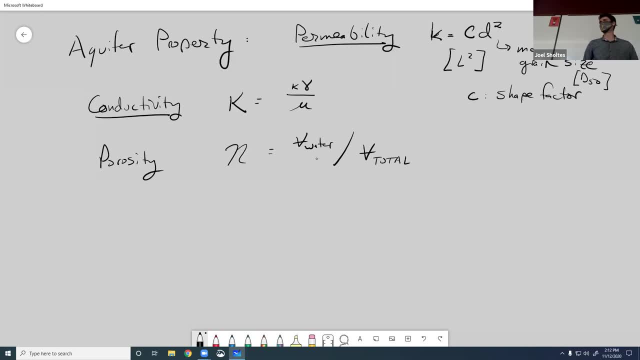 Unless she hasn't been texting me, because all the cell flow and towers have blown out. I had to be breaker. Okay, I don't think. I think it's okay. um, all right, no, I think it's. I think she would have. I don't know. there's a lot going on, so maybe you can. 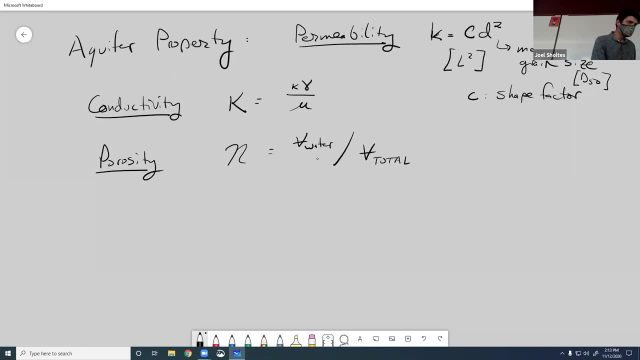 like ignore the fact that it's almost December and there's a hurricane barreling down on you all right. and then we introduce Darcy's law, which says that the discharge in an aquifer is equal to negative hydraulic conductivity times, area multiplied by the gradients and head. 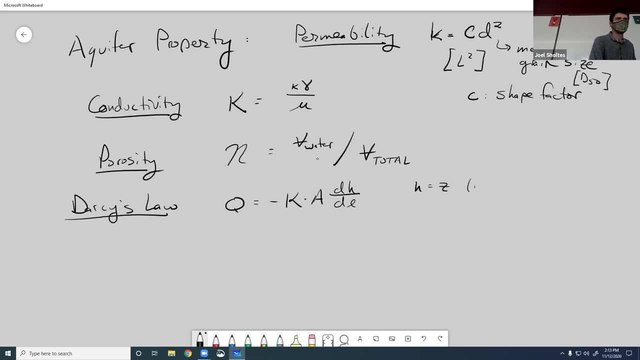 where head is defined as the elevation of the water table, z for an unconfined aquifer, and head is equal to the z plus pressure over gamma when we're dealing with a confined aquifer. and the way we might think about Darcy's law is: if we have 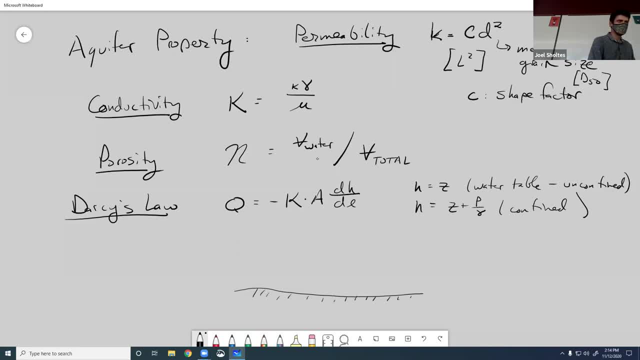 some aquifer that has some thickness to it. that's the bottom of the aquifer. um, here's the ground surface. here's our water table. sorry, it's hard to draw straight lines here. and if we look at the slope of that water table for an unconfined aquifer, we put a well in here. 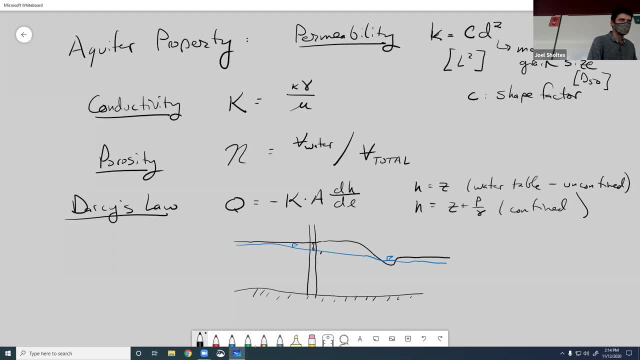 and we get the depth. or we could also think about it as the elevation from the bottom of something. some arbitrary elevation Say this is h1 and h2. And then this is our length. Then, in this case, our gradient is going to be delta h over L. 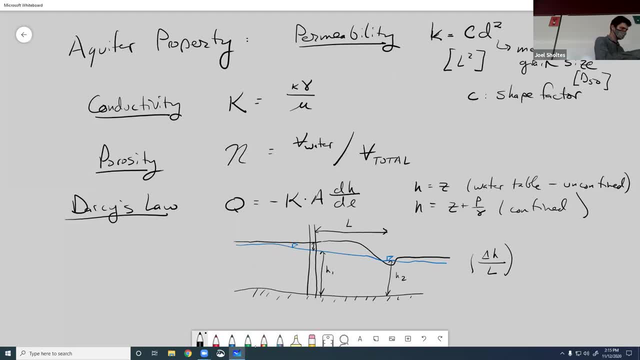 Right, Well, delta h would be negative. Yeah, Yeah, Hey Joel. Yeah, So is permeability like lowercase k and then conductivity, uppercase K, Correct? Yeah, and I don't think we're going to be calculating permeability directly. 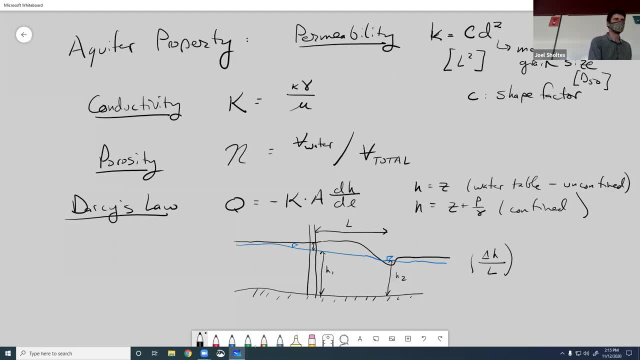 I just want you to know that conductivity is a function of the permeability and the properties of the fluid, And I should note that the units for conductivity is length per time. Okay, So let's talk about transmissivity and we'll do an example calculation. 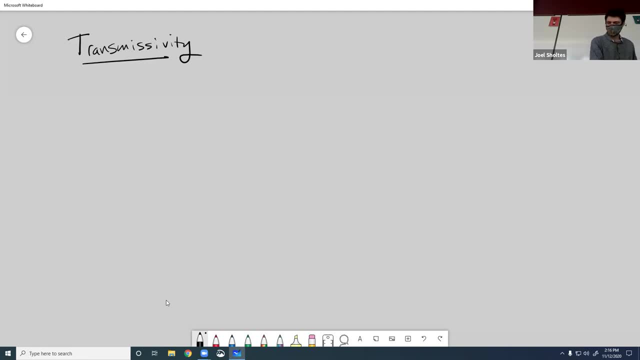 All right, So let's talk. first, Excuse me, Let's look at a little slice of an aquifer. This is kind of like a piece of cake Right here, And, trust me, transmissivity is a piece of cake. 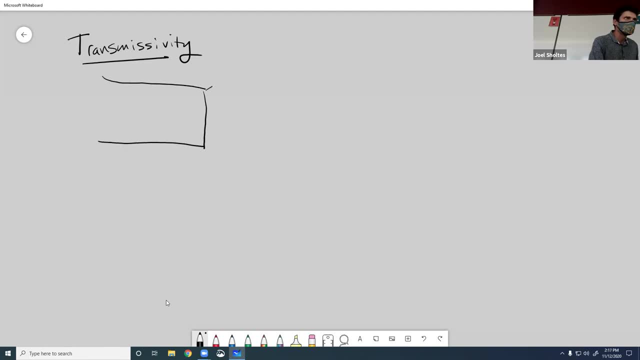 But we'll look at a piece of cake. So this is the bottom of our aquifer. This would be like an aquitard bedrock, some impermeable layer. We have the water table in there. This is an unconfined aquifer, right. 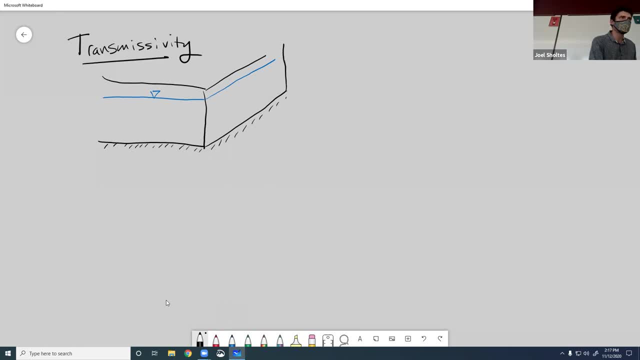 Let's actually put a bound here and give it an actual width. B is going to denote the thickness of the aquifer up to the water table, And then for transmissivity, we're interested in kind of how much water is flowing through a unit area of this aquifer. 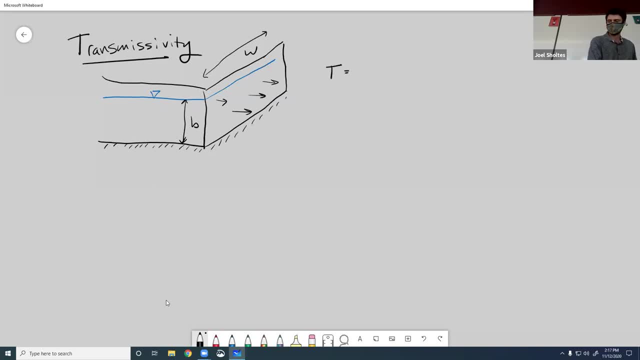 T is equal to the big K times little b. in this case It has units of length squared per time. Okay, So this is going to denote the length of the aquifer. Okay, And so W is really just a unit width. We'll get at that in a second. 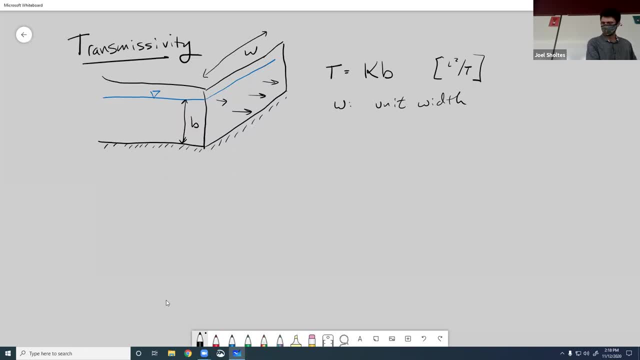 Big K Hydraulic conductivity, And we might just assume, based on the quality of the aquifer, We can say K is equal to some value. In this case we'll just say it's 50 meters per day. We'll go back to the Darcy's equation. 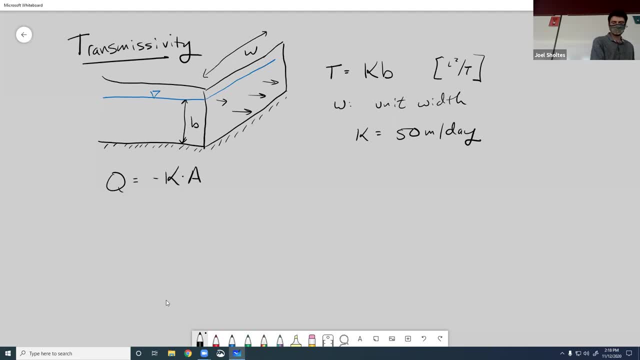 Q is equal to negative big K times, area times the hydraulic gradient A is equal to B times W. Okay, So I'm just substituting BWN for A right here, And then, because transmissivity is equal to K times B, Then we can say this is equal to negative T times W times DH over DL. 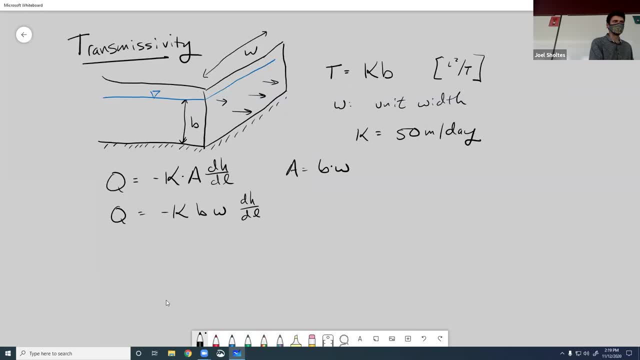 Okay, And then we can say this is equal to negative T times W times, DH over DH. So ultimately we can calculate transmissivity as our, as a property of all these parameters. So if we solve for T in this case, We can get: T is equal to the unit, the discharge per unit width. 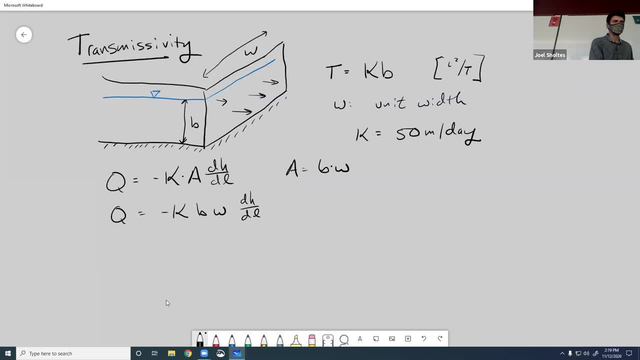 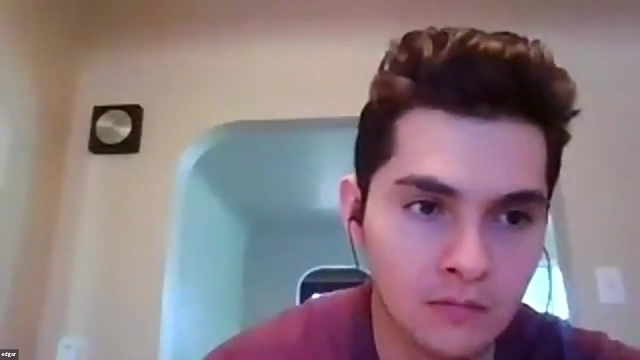 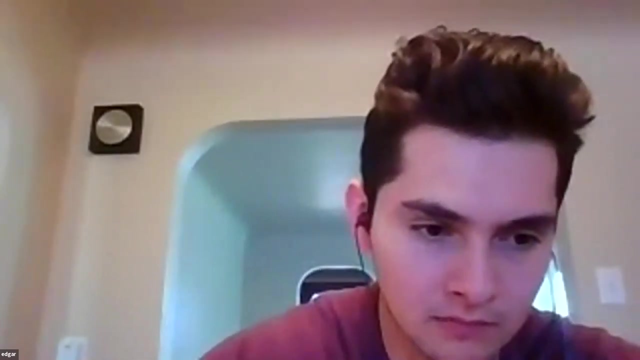 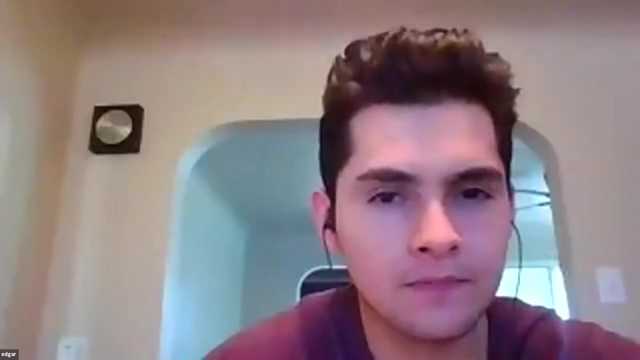 So Q divided by W Times, the hydraulic gradients, The inverse of the hydraulic gradient, DL over DH, And so this is the kind of The whole definition of this is how you might calculate the transmissivity Of an aquifer. Okay, 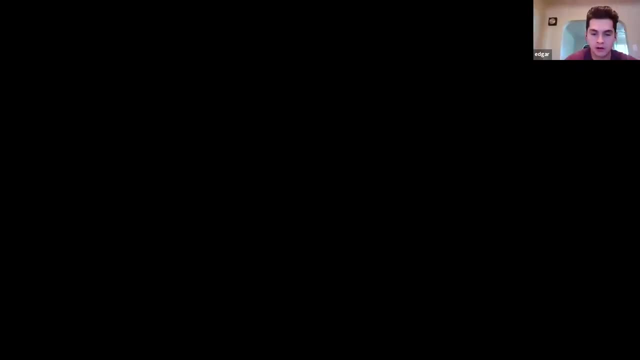 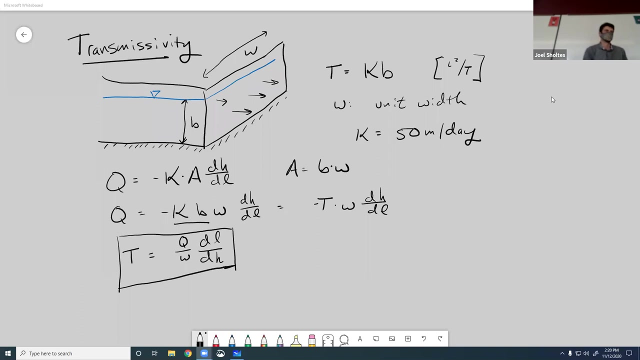 Are we still recording? Okay, Yeah, You're good now. Okay, great. What does transmissivity tell us about an aquifer? Yeah, How much. how much flow is moving through it, How much water you can kind of move through this aquifer. 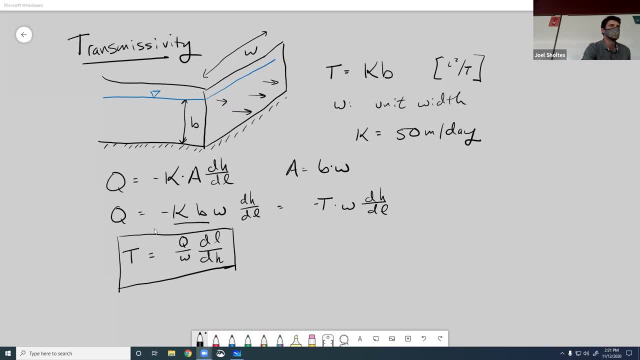 It's going to be a function of the hydraulic gradient. We can- we can- calculate the flow. Now we can actually do a calculation And so make some determinations of discharge and an aquifer And actually get an idea of how How much water is flowing through an aquifer. 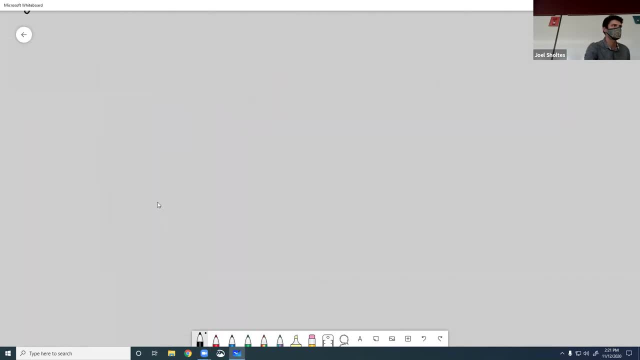 Let's do a calculation. Yeah, Yeah, Yeah. so you're assuming B doesn't change over time? Yeah, that's an important assumption. I guess a couple other you know. let's talk about assumptions. I skipped those Engineering problem solving right. All right. so assumptions: this is steady state. 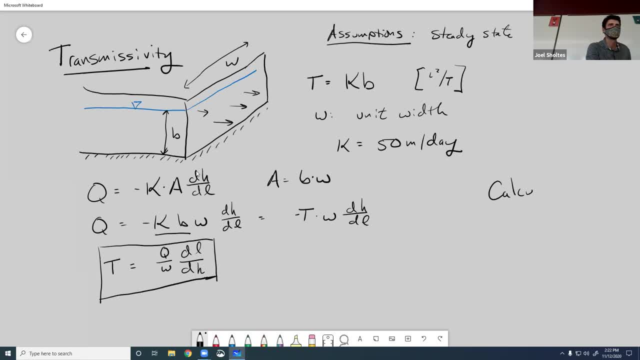 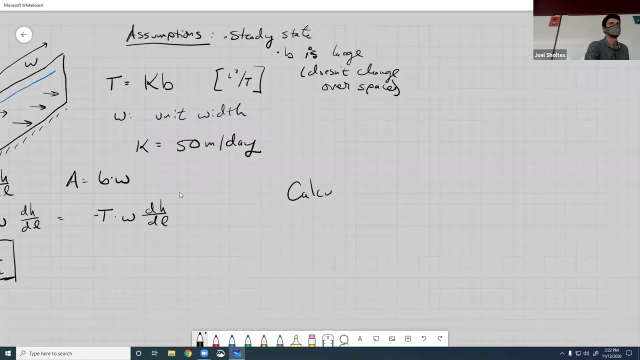 B, meaning the discharge isn't changing over time. And then B is large, meaning it's not changing a lot over time or over space. Let's calculate, let's do an example. We're going to calculate T and K, So we'll look for this example. We'll have some idealized aquifer, an unconfined aquifer. 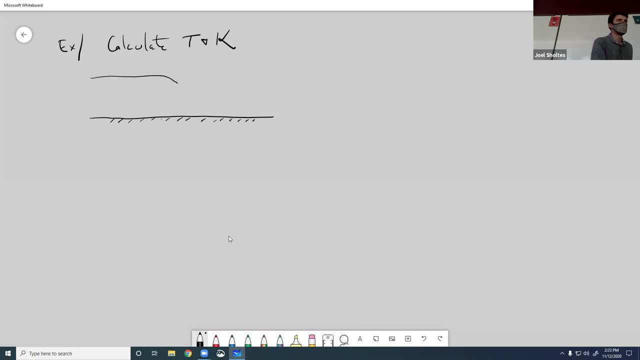 And we've got kind of a valley going down to a creek or a stream. It comes back out And we've got a well. It goes down and where you can observe the depth of the water, we'll say it goes all the way down. 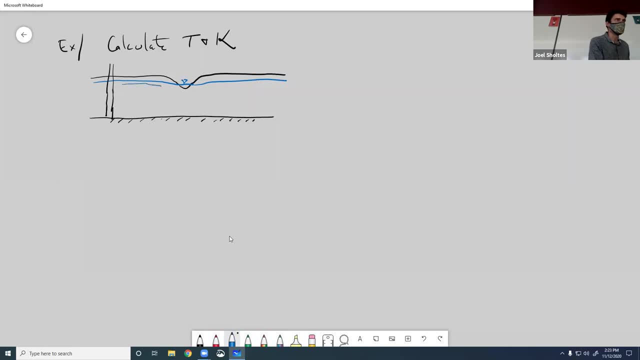 And the flow path for this water, this groundwater, is, you know, it's kind of going downhill towards the creek right. This creek also kind of goes back into space, So it's got a length associated with it And we'll say that. 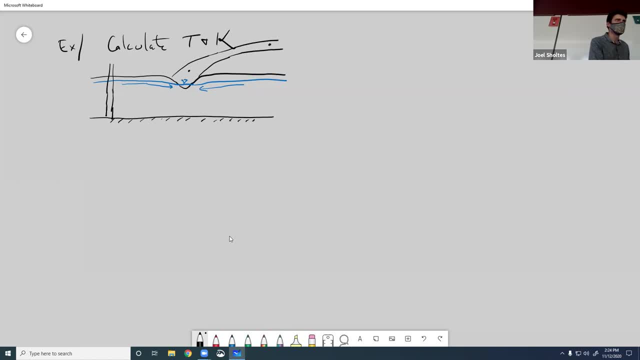 We'll kind of run it over here. We've got two observation points where we're measuring discharge, And between those points we have 5,000 meters And The thickness of the aquifer is 50 meters, And then from the well to the water surface, 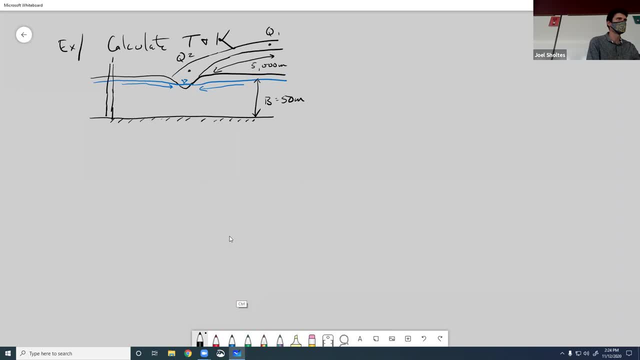 Let's just. Let's just draw it down here, Just getting a little cluttered. The length is 2,000 meters, or dH is one meter. So you can imagine a situation where we've got a creek. we can measure the stream flow through. 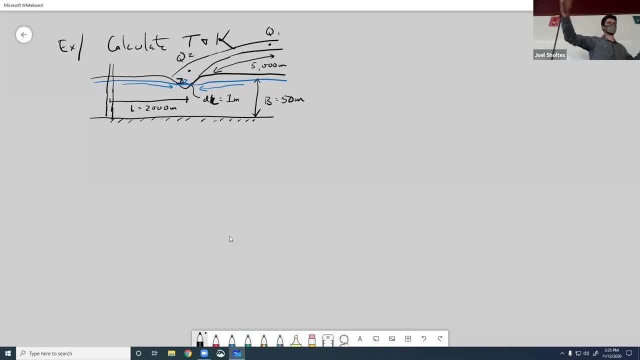 that creek over a kind of valley that has like a homogenous type of aquifer material in it and we can take observations of the discharge change under base flow conditions, so no surface runoff between these two points, and then we can have an observation well nearby and try to get an 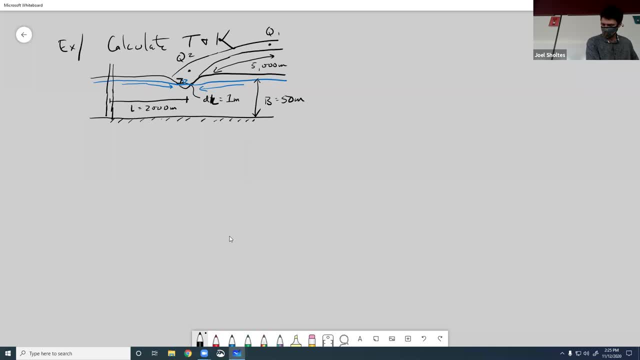 estimate of the hydraulic gradient between of the water flowing from the valley margins to the creek or the stream. All right, so we have two stream gauges and at point one we have measured 2.355 cubic meters per second, and at the second stream gauge we've measured 2.485 cubic meters per second. 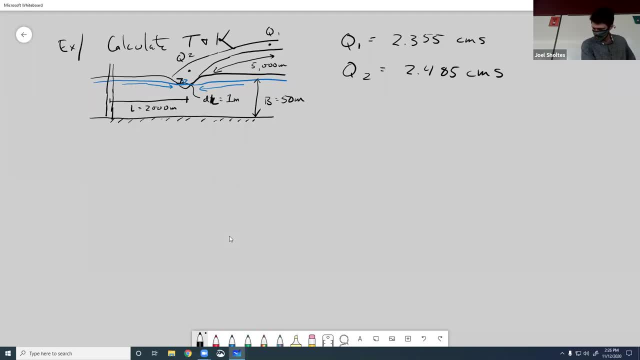 All right. so we got a little bit of an increase, right. And our delta Q? in this case, we just do the subtraction as or the difference. there we got 0.130 cubic meters per second. That's our delta Q and that's over that 5,000 meters, right. 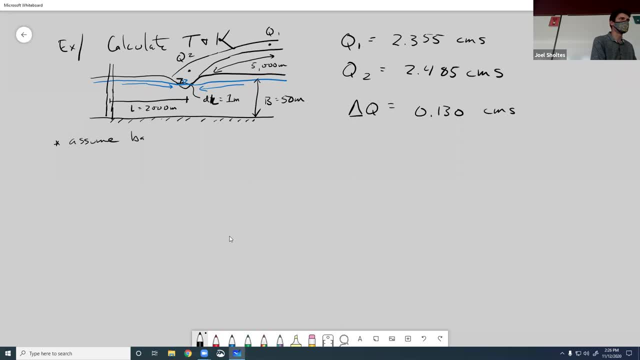 So first we're going to assume we're under basal conditions. yeah, What's that? what's what's dH? real quick, What's a dH? So dH is that's one meter, but like, yeah, so it's the change in elevation. I didn't draw it super well. 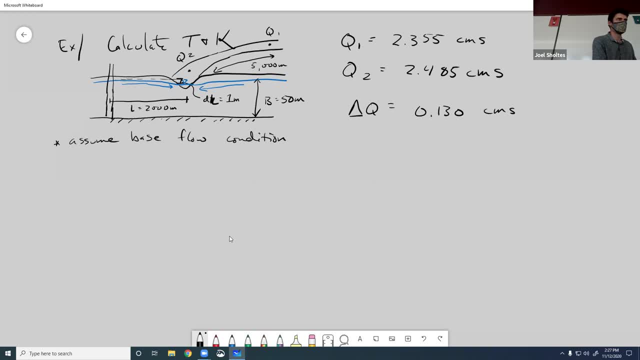 here. it's the change in elevation from this observation well to the water surface in the creek. Does that make sense? It's the gradient, it's the overall slope of the water table from that observation well to the creek. Okay, okay, it makes sense. thanks, yeah. 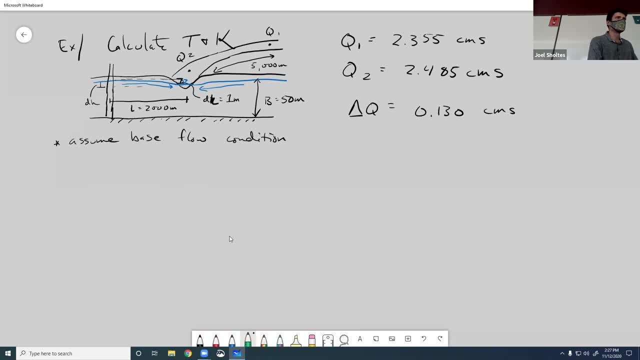 All right. so what we're going to do to solve this problem is we're going to basically draw, cut this problem in half, because we have water flowing from this side. we have water flowing from this side and we're going to assume that the water's flowing at an equal rate. 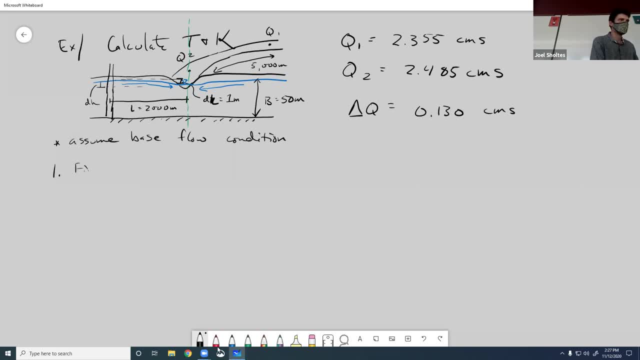 we'll do is we'll find the inflow to the stream from groundwater between points one and two and then we're going to divide by two, because we're going to assume that we have equal contributions from either side of the valley or either side of the stream. then we'll convert. 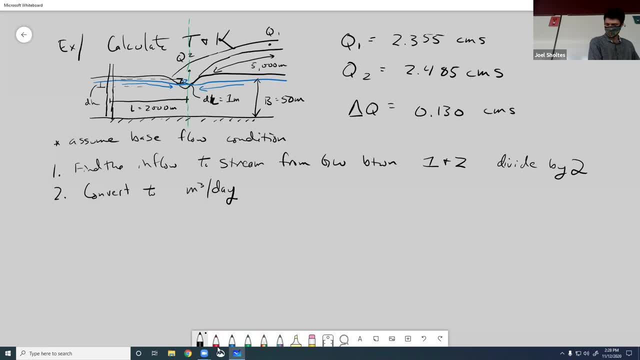 to cubic meters per day. this is the kind of the units of k. if we did it per second, it's going to be a really teeny tiny number. so let's go ahead and convert the cubic meters per second. so we want to divide this by two, remember? 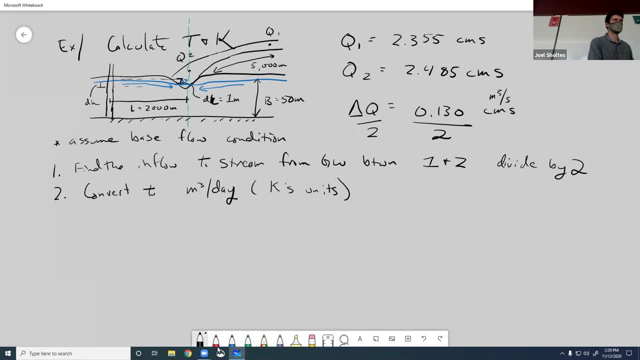 convert two cubic meters per day. yeah, and then we'll go back to that transmissivity equation. all right, so how do you guys do that? for the next two minutes, all right. so let's go ahead and convert the cubic meters per second. all right, so I want you to do that conversion. 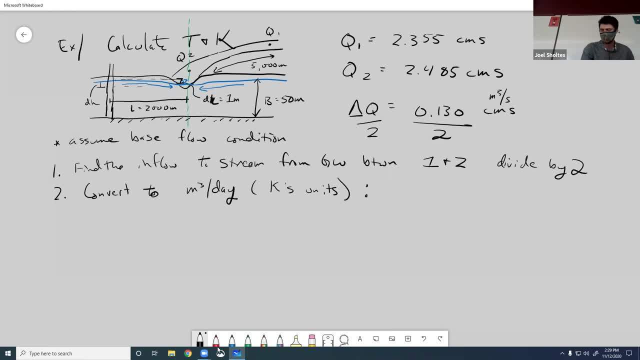 and I'll write it out here slowly. so we have 0.065, is that right? so 0.065 meters cube per second times 86 400 seconds per day. 0.065 meters cube per second times 86 400 seconds per day. 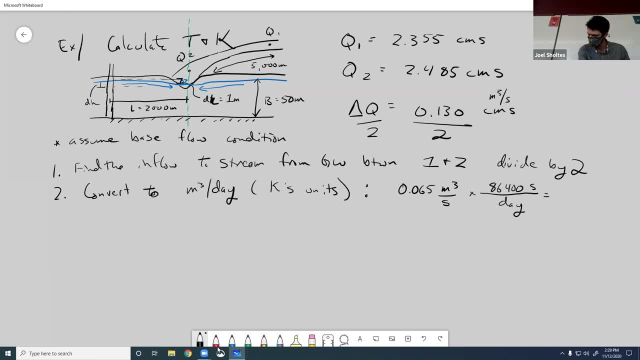 0.065 meters cube per second, times 0.065 meters cube per second times. times times, T is equal to 5,616 cubic meters per day. Thank you, Agar. All right, Now we'll go back to our equation. for transmissivity, T is equal to the unit discharge. 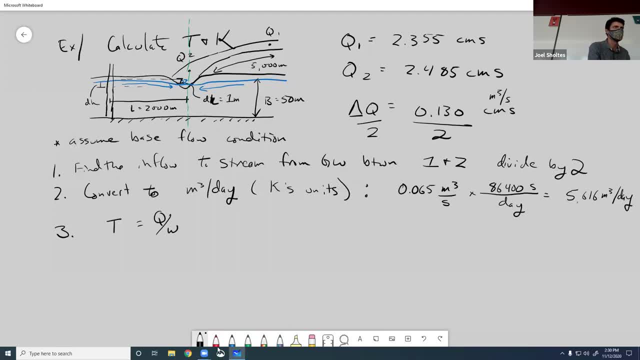 the discharge per unit width. In this case, we know the discharge that's coming in over that, 5,000 meters times the inverse of the hydraulic gradient- dL over dH- And so all we'll do is plug in those numbers: 5,616 meters cubed per day, And that's going to be divided by 5,000 meters. 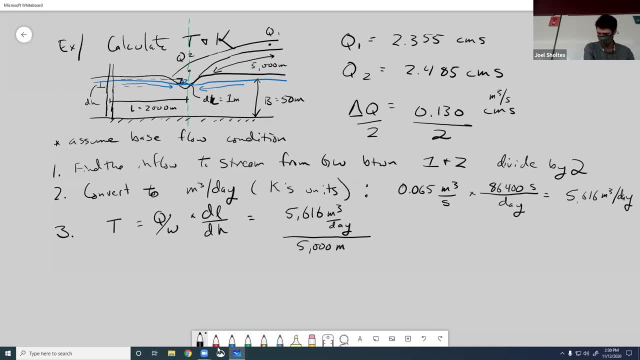 which is our W, And then we'll multiply that by our dL over dH. Our dL was 2,000 meters and our dH was 1 meter, So we end up with meters squared per day, which is the unit's length squared per time. 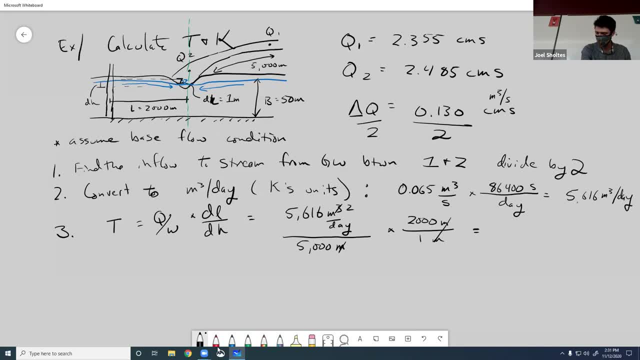 of transmissivity. And if we do that calculation we get T is equal to 5,616 meters cubed per day, And then we'll multiply that by our dL over dH, So we'll go back to our equation for transmissivity. Now we're going to plug in those numbers. 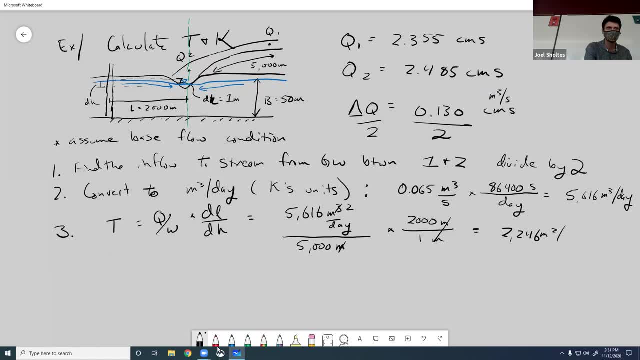 And then we'll plug in those numbers, Keep doing the math, And then we'll plug in those numbers. And then we'll plug in those numbers our aquifer depth, which was 50 meters, And that gives us a hydraulic conductivity of 45 meters per day. 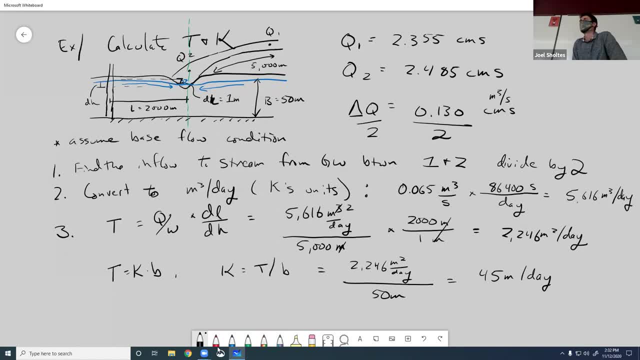 So this is actually something you could do. You could measure flow rate. Flow rate is hard to measure in surface water. It's hard to really measure anywhere, So you have to have a really precise way of doing that, And the best tool we have these days. 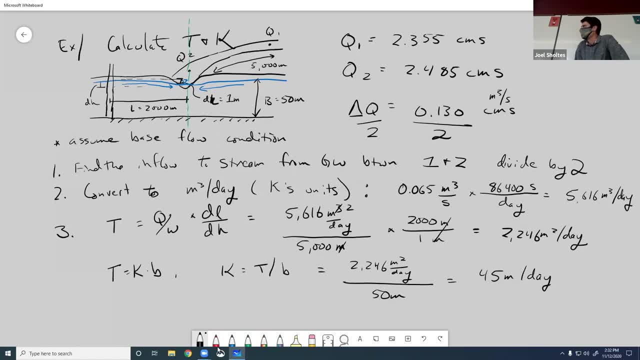 is called acoustic Doppler profilers And they're able to give you usually their boat mounted or even a raft mounted And they're able to basically tell you the velocity of these cells in the river, the two dimensions of that cross section, And they give us the most accurate estimation of discharge. 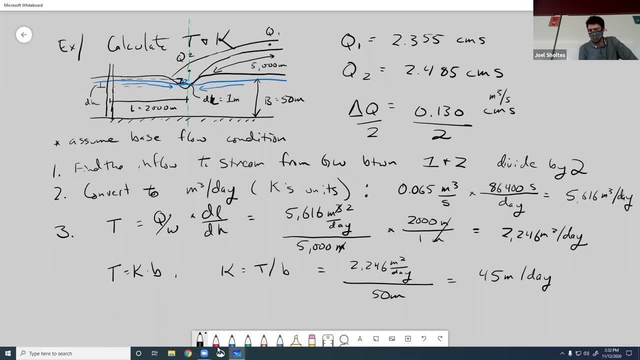 So we could use some really precise instrumentation to do that. You could have a flume upstream and downstream- Sometimes in research areas we use flumes to get that difference in discharge- And then you could have observation wells and then you would get this transmissivity. 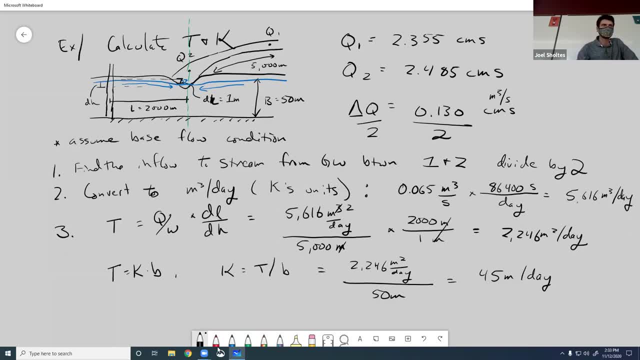 and hydraulic conductivity. We used weirs. you can use weirs right to calculate discharge. A dam like that, certainly you know you could come up with a weir coefficient for it. So, yeah, really any kind of hydraulic control. 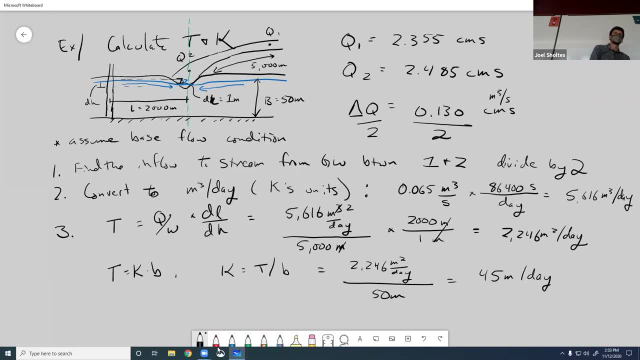 can be used to get a better representation of discharge. All right, All right, That is. That's our first calculation. We're 30 minutes in And I think I'm going to do one more, and then we'll take a quick little brain break. 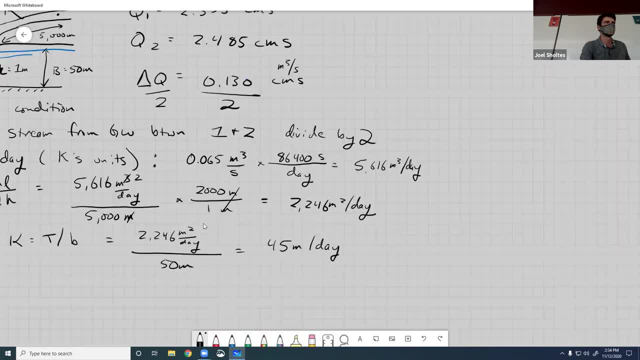 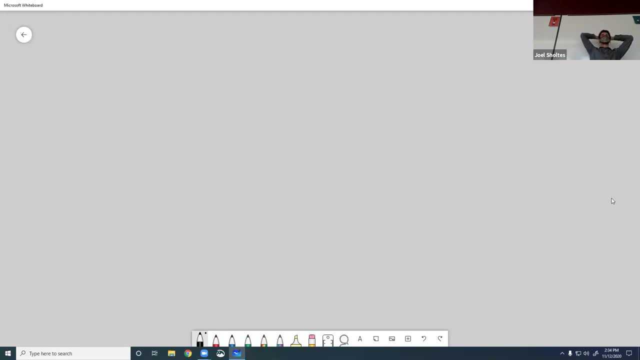 What do they use to split the water from the south or the lower basin? how do they measure that? The stream gauge, Yeah, So the way a stream gauge works is The stream gauge that they use. Yeah, Do you know how that works? 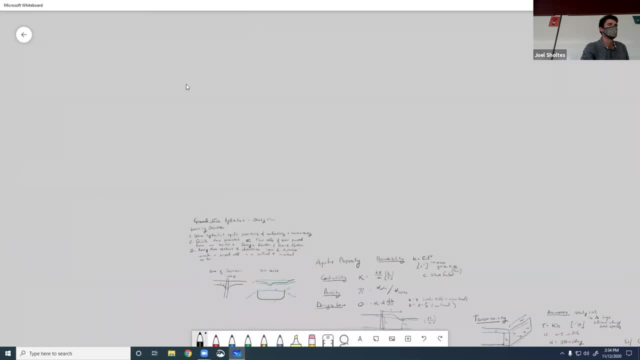 Yeah, Okay, We'll just, We'll do a stream gauge real quick, Hey, Joel, really quick. Yeah, That last example, that was a confined, Unconfined. It's like confined to where we're like pressurized. 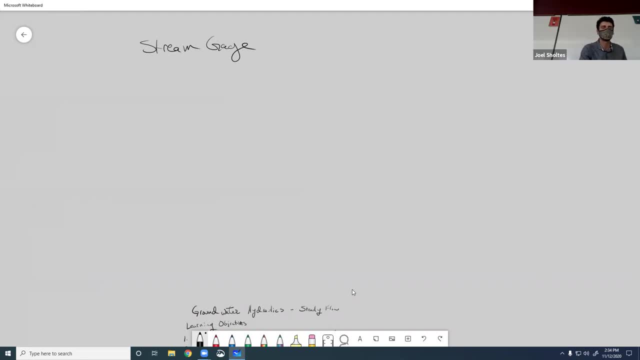 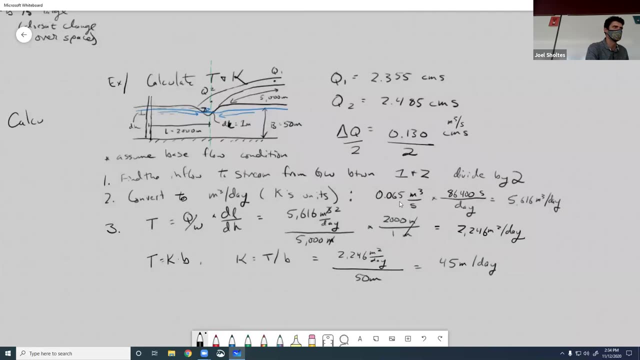 Not pressurized. Yeah, Not pressurized. Yeah, Let me. Let me try to try and see if it works. It should be in base flow conditions and then, And if we do have a confined aquifer, we would draw that confining layer. 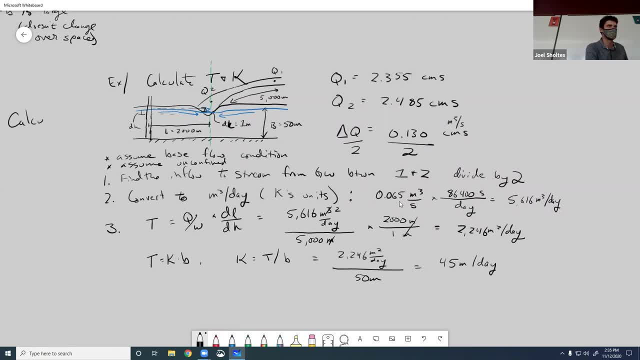 so it'd be really obvious In this case. you can see that this water table surface- you know I drill out a little triangle. that means it's a free surface. There's no pressure acting experiences on that Okay, other than atmospheric pressure on that surface. 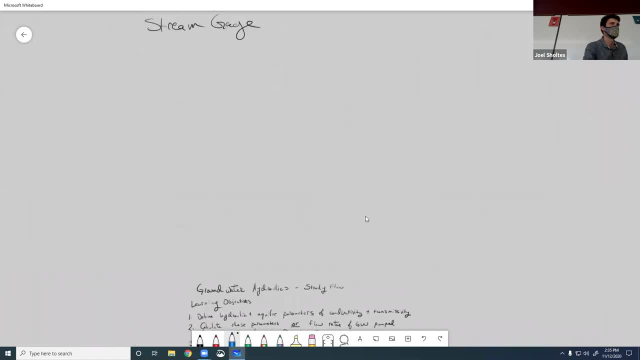 Thanks for that clarification. Real quickly about streamgages. The way streamgages work is they measure something that's easy to measure. Here's a little streamgage house- Maybe it's like a corrugated metal pipe and they put some data logger in it- and what they're usually measuring is: 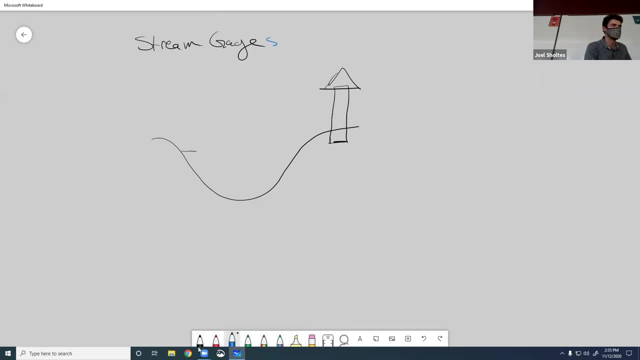 well, I guess we'll just do it the most simple way. There's a lot of different ways they can measure the stage of the water. The most intuitive way, I think, is just an acoustic sensor like a Doppler. It sends a ping down and then that ping comes back. 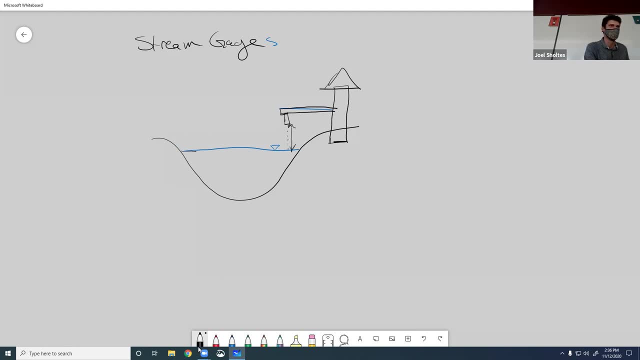 It's able to tell you the distance of that water, the elevation of the water relative to some datum. They'll have some surveyed benchmark. The surveyed benchmark has a certain elevation associated with it. Then we can get the elevation of the water relative to that datum. 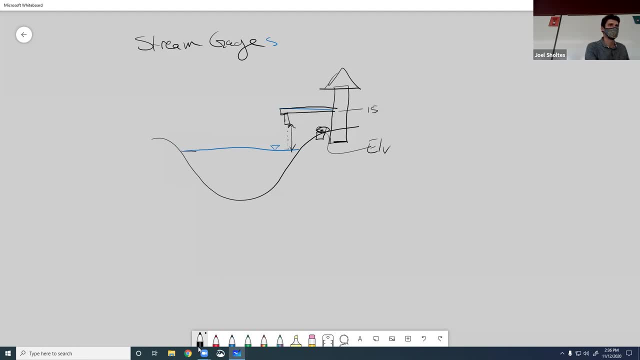 This is easy to measure and we can measure that every 15 minutes or something like that. Just the elevation of the water, of the stage That tells you a flow, because you're having cross-sectional areas at that point, The way you get to flow is you basically are just doing. 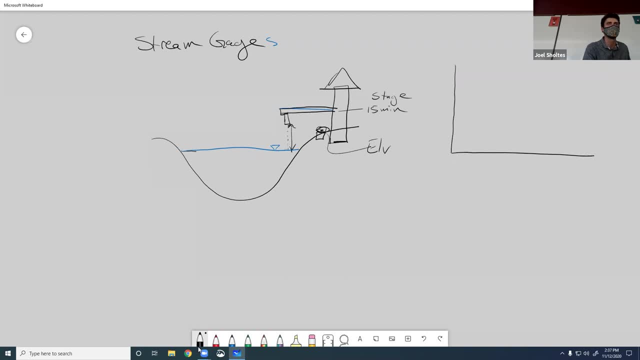 a statistical relationship and empirical relationship between stage and discharge. Typically for a rating curve, we put stage on the y-axis, But in linear regression, stage is going to be our independent variable and discharge is the dependent variable, the one we want to try to predict. 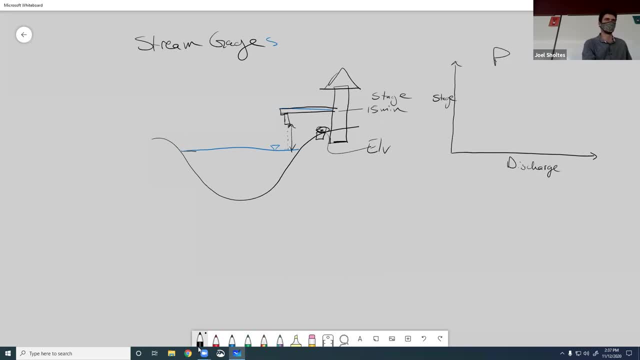 Usually that goes on the y-axis, but this is the way we visualize rating curves. You have to develop a rating curve and each USGS gauge has a rating curve that's developed from point measurements where they'll go out in a little boats or maybe they have. 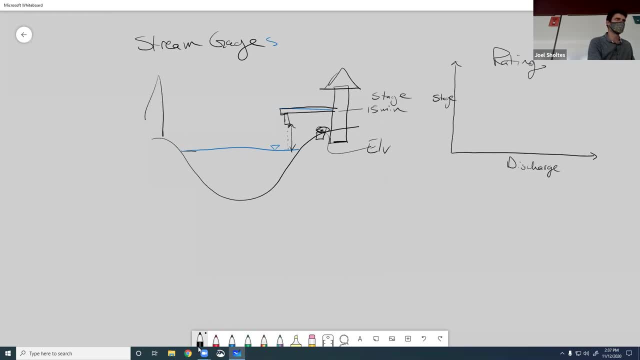 sometimes you'll see these tramways that go across a little cable car. Then they'll sit in that cable car and they'll put down a device that can measure the velocity of the water, or they'll get in a boat and put their acoustic Doppler velocimeter in there. 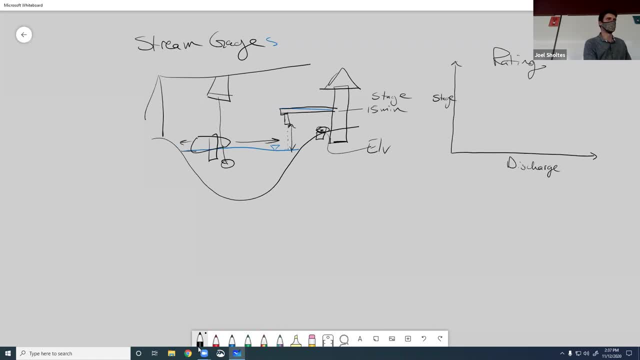 and just go back and forth. They take velocity measurements across the channel. They know the depth of the water because they know the cross-section shape. or maybe they measure the cross-section shape every year or something like that, because it's going to change. 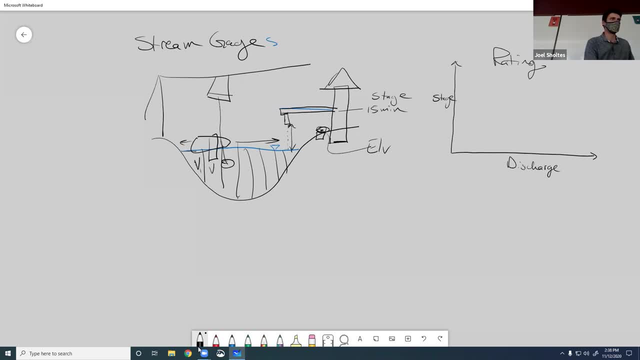 If you add up all these velocities and areas, you get the discharge Each time they go out there and they'll go out there many times a year. there's a whole host of hydrologic technicians that go to all the USGS gauges and they take their measurements. 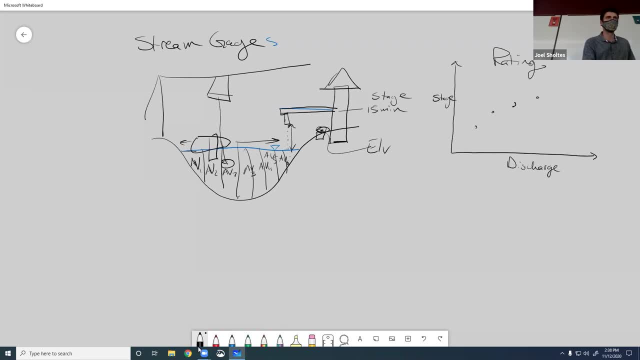 They get a bunch of points Over time and they fit a curve which is just an equation. Q is equal to some function of stage. That's a rating curve. That rating curve is always being updated. They're going out and taking their measurements. 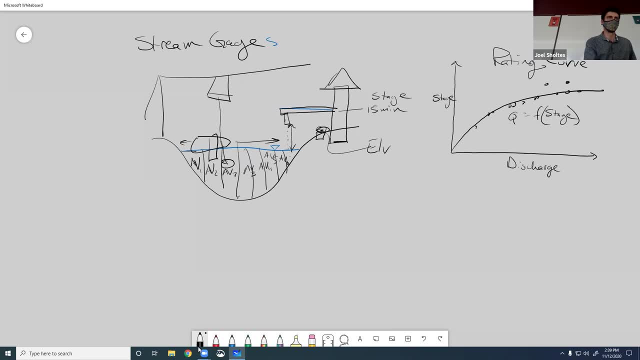 and all of a sudden, if they get a couple of points over here, they're like: oh, we got to shift the rating curve. They document all that stuff. You can go to any USGS gauge and download the rating curve. It's data that they have up there. 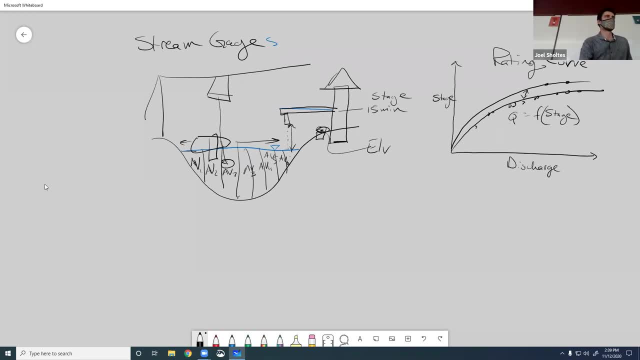 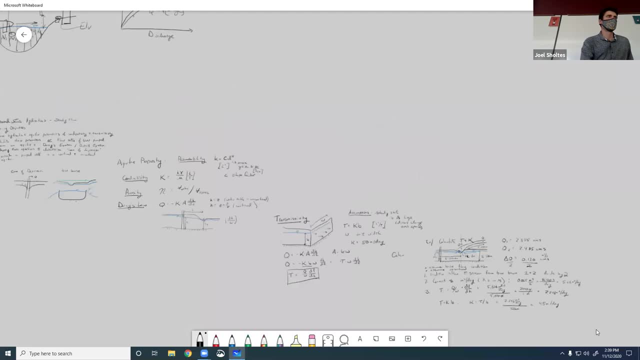 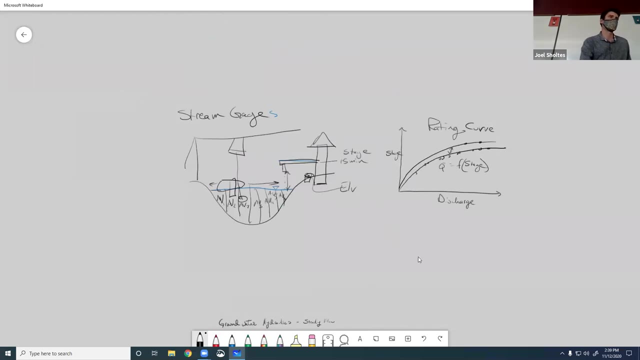 and that's a document every time they go out and take a measurement. It's really hard to do in natural channels. It's hard to do well. That's why you have to have really sophisticated equipment in. USGS is the best equipment basically. 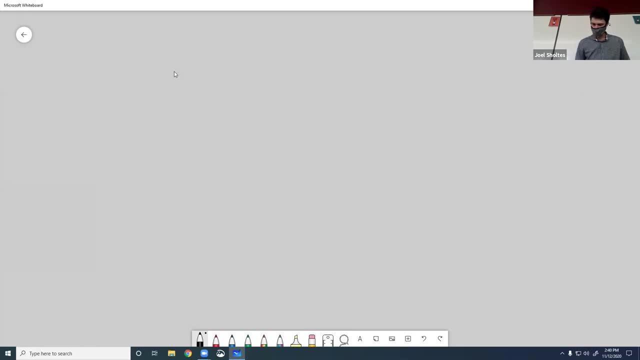 All right, let's do one more setup here and then we'll take a little brain break. We're going to talk about Dupuy's equation- Again, sorry for the butchering, And again this is for steady state flow And really this is just another way. 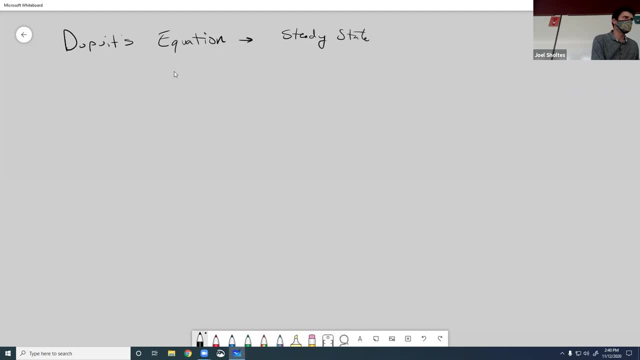 of writing Darcy's equation, but we'll kind of. but it's how we think about how we might actually measure hydraulic conductivity or groundwater flow, based on observations from two different wells. So here's our ground surface. We'll have one. well. 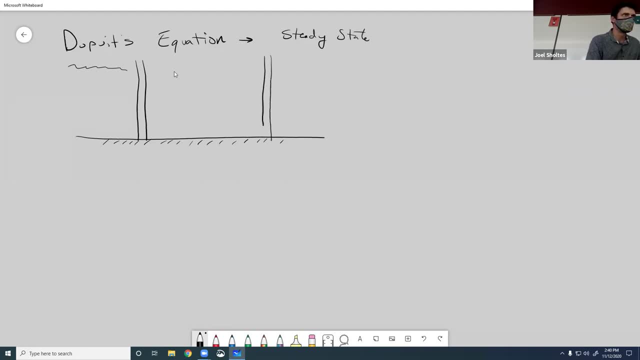 then we'll have another well, Have our water table, and the water table is going to be sloped Like this. it's a unconfined. Right now it's unconfined, but this works with confined. This is unconfined. 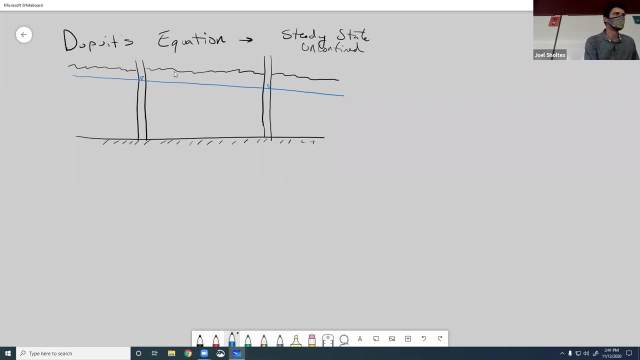 And water is flowing in this direction And the ground surface is unconfined, All right, So we're actually going to have a little bit more damage to the ground surface. So what we want to do is we want to pay attention to the ground surface. 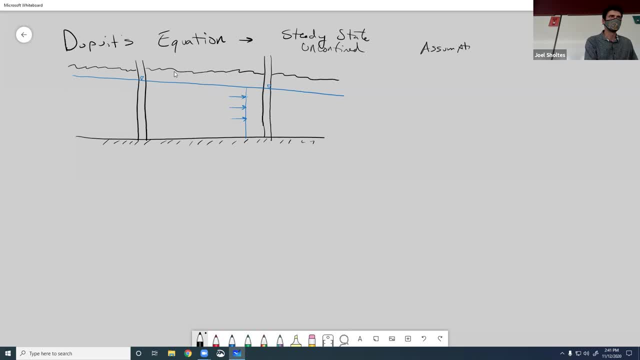 We're going to look at the ground surface and we're going to measure the surface. So I'm going to really just use a pebble and we're going to measure the ground surface by measuring the surface. All right, All right. so let's just list out the assumptions here. 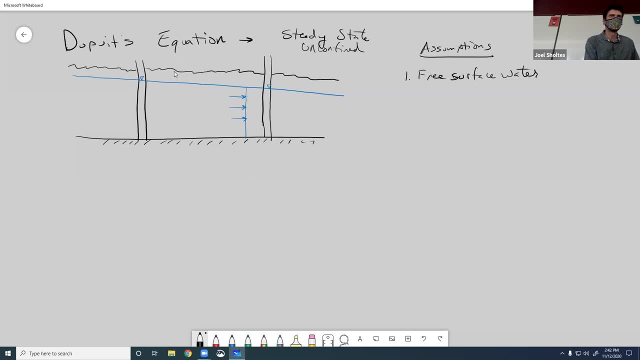 So one is, we have a free surface water table, which really just means it's unconfined. So this is our ground surface. We can just zoom in here and see what's happening. So here's a little move over here. All right, All right, And we're going to measure. 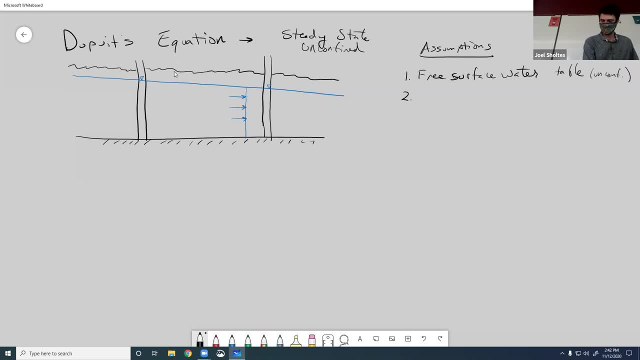 We have a very small slope or hydraulic gradient. This is kind of similar to when we did open channel hydraulics and we said that the gradients is small enough that you know things are transitioning smoothly over time. we don't get like turbulence or bending flow lines and that sort of thing. 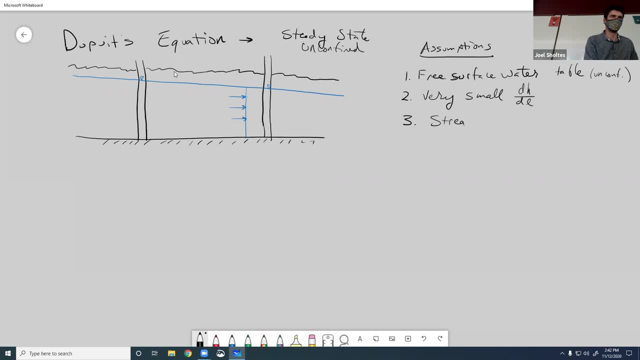 So this also means that the streamlines are parallel. Streamlines are parallel to each other, so streamlines are just. if you were to put like a dye in the water, that dye would slowly make its way in a parallel fashion with any other point of dye that you would introduce into the aquifer. 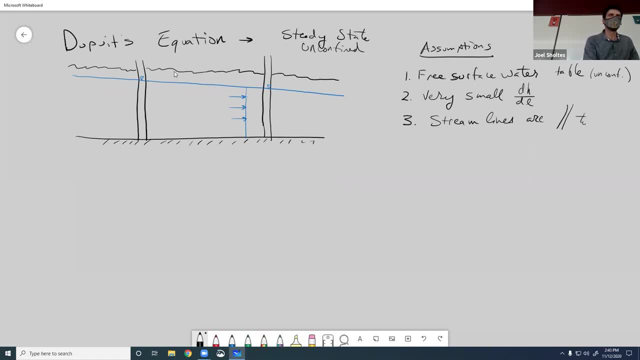 So they're parallel to the water surface And that's streamlines are symbolized by the symbol psi, And then equipotential lines, Okay, Symbolized by phi, are perpendicular. And so if this, if these lines right here, are psi, then the, this would be an equipotential. 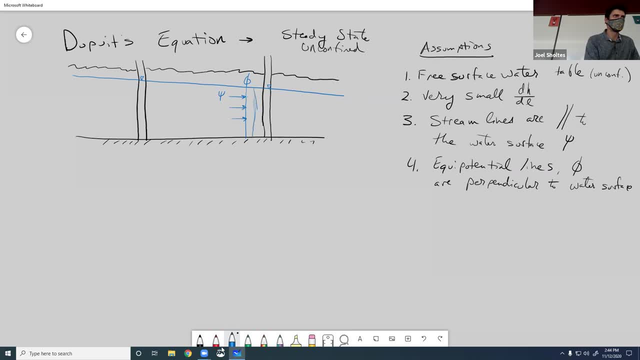 line. All right. and then the last assumption here is that the friction slope. the friction slope is equal to the actual slope of the water, So this is uniform flow, and we saw this in open channel hydraulics. Okay, Okay, All right. 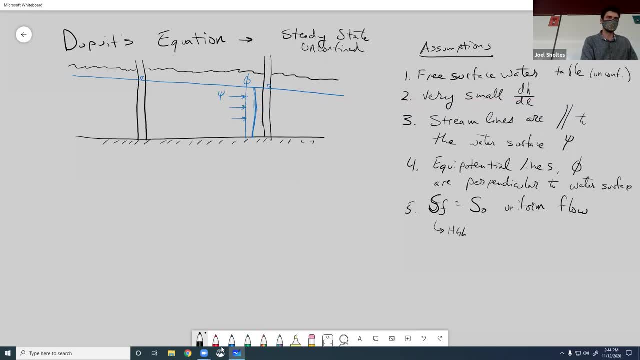 This would be the slope of the hydraulic grade line And this is the slope of the water surface. Hydraulic grade line is just the the. it's going to be equal to the water surface for an unconfined aquifer. All right. 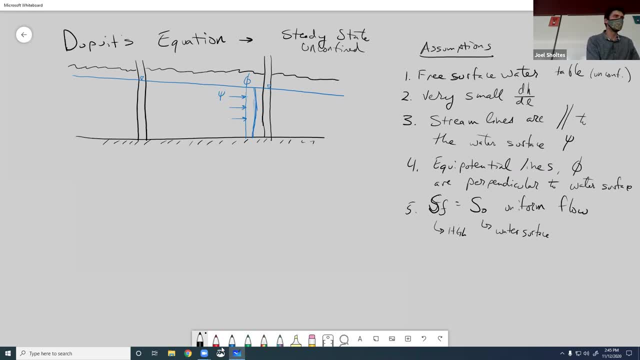 If we Okay, So we're looking at this aquifer kind of a two dimensional slice. Now the aquifer we could imagine extends out into space at some unit width. We're not going to define what that is, but we're going to put this equation in terms 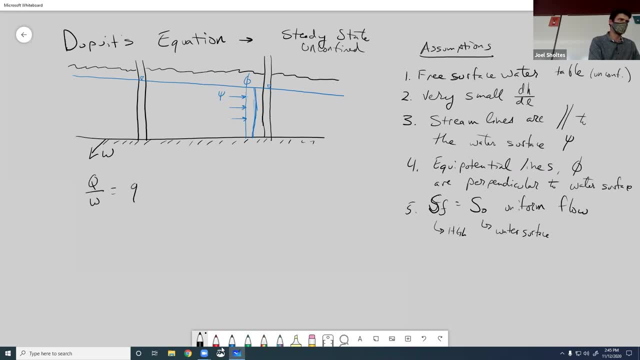 of Q over W is equal to lowercase Q, which is just discharge per unit width of aquifer, per unit chunk of aquifer, And we'll go back to our Darcy Okay, And we'll go back to our Darcy equation and say that this is actually well, first needed. 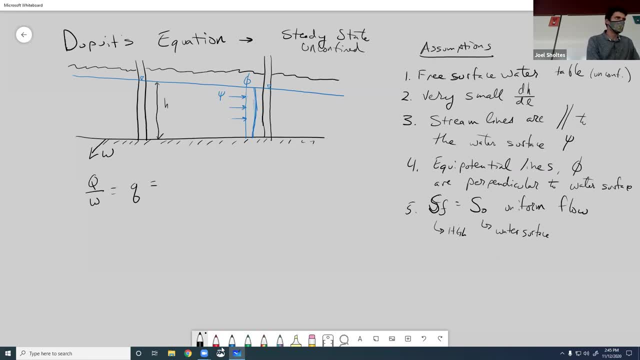 to find a couple of things. The height of the water table above some aquitard or some impermeable layer at this point is going to be H naught. So this is going to be zero and the X direction is in this direction. 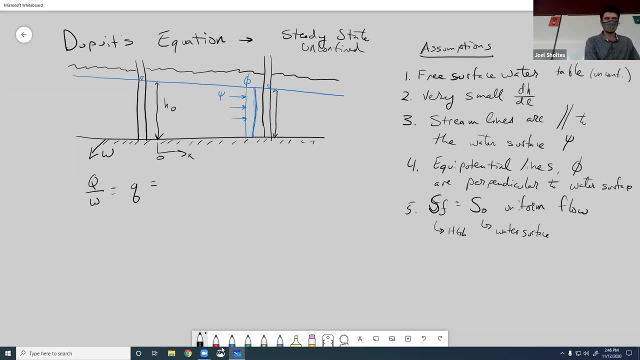 And then the height of the water table at some point downstream It's going to be H X H as a function of X. All right, So back to our Darcy's equation, for when we do the lowercase Q here per unit width, we 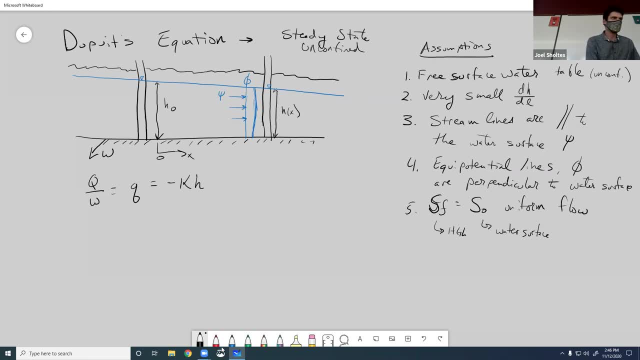 divide it as K times H, D, H over D, X, where it used to be area here. but we divided by W. So the depth of the water table times the width of the aquifer would be area, right. So we just took that W out. 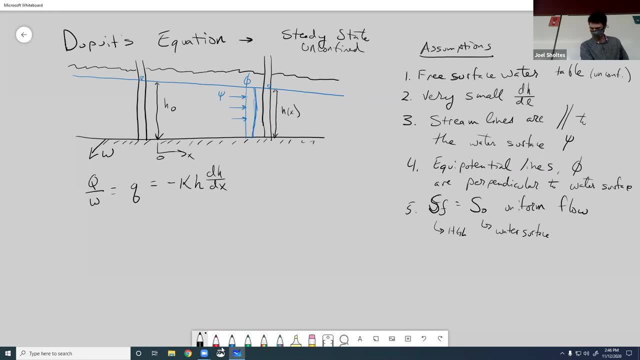 So H is just the depth of the water table. So there's a derivation here and I'll post my version of it on Canvas. It's also in your book, But we're going to save it, We're going to skip the derivation and we're going to say that based on two observations. 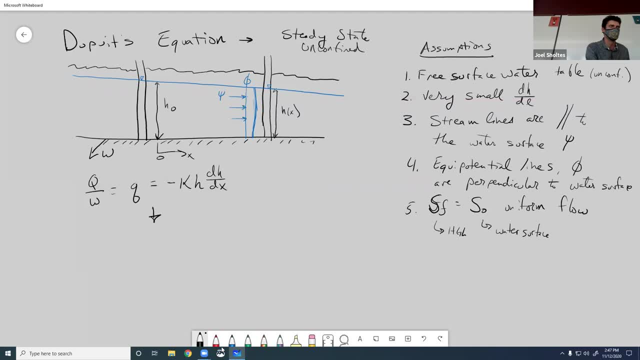 of the water surface depth from one point to another at some distance L. so two observations of water table at distance L, Then the discharge can be related to those observations and the hydraulic conductivity. So K over two L times H, knots squared minus H L squared. in this case X is equal to L. 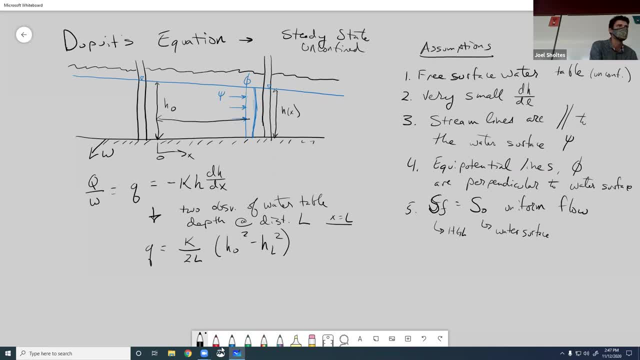 So just some distance between this observation and that observation. Okay, All right, All right. So what this does is this describes the water table surface as a parabola And this, ultimately, is what's going to lead us to the cone of depression calculations. 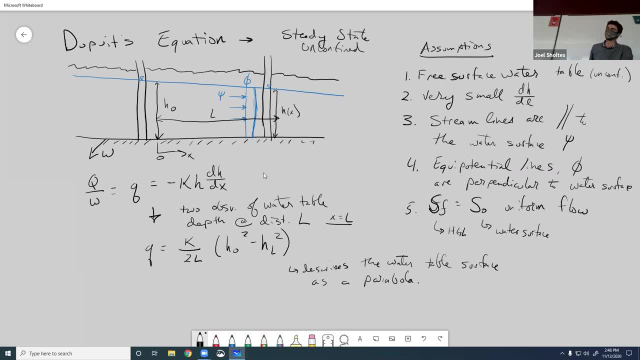 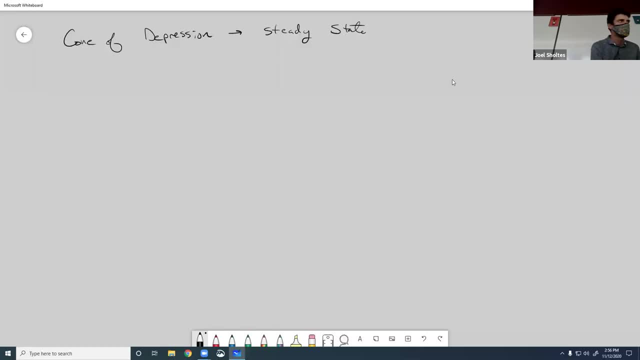 that are kind of the bread and butter. So this would be the question of FE level groundwater hydraulics. There we go. Val and Edgar, are you guys on? Okay, Hopefully that's a yes, Val and Edgar, are you guys on? 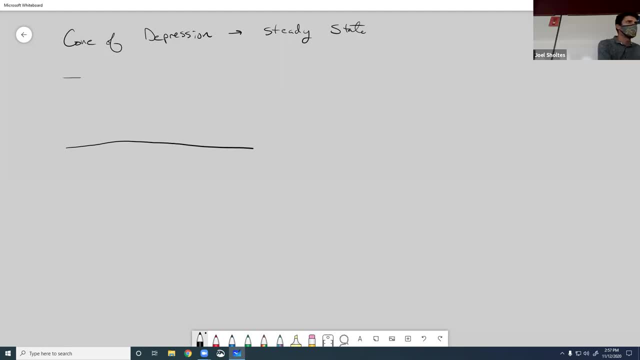 Okay, Well, I'm recording it So you can look at this We have. so we'll just kind of we're drawing a lot of these cross sections here. So first we'll do an unconfined aquifer And we'll have a well coming down. So in this well we're pumping water out of the well. 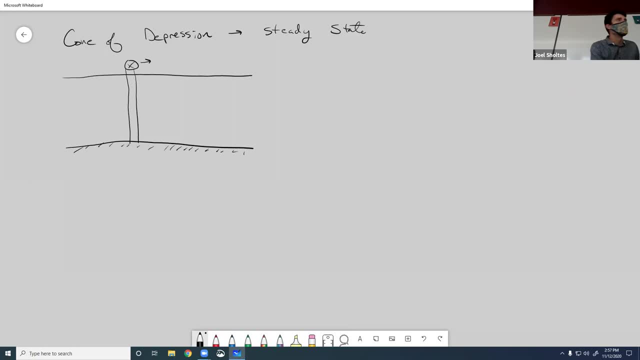 So we've got a pump and there is a flow rate big Q coming out of it And we're pumping so much water that we're getting a cone of depression. Now this, of course, is really exaggerated. right, We talked about the slope of the water surface not being very great, So we draw this in a very exaggerated. 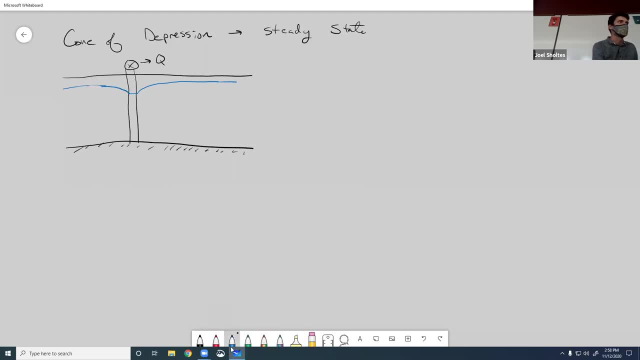 manner. This might be, you know, a drop of a foot over thousands of feet, or something like that. All right, and then we can have another well, and that could be a well nearby, Or it could also be just a well, it could. we could be doing this calculation between two wells. 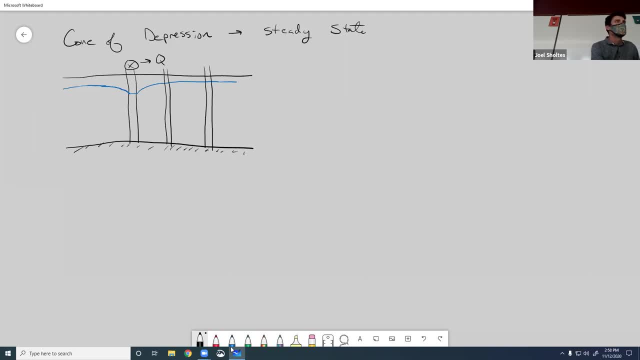 This is just. this would just be two observation wells, right, The pumping is happening over here and then we have two observation wells. You just need two wells, either the well itself where the pumping is occurring, or two wells nearby, so you can get that slope of the water surface. 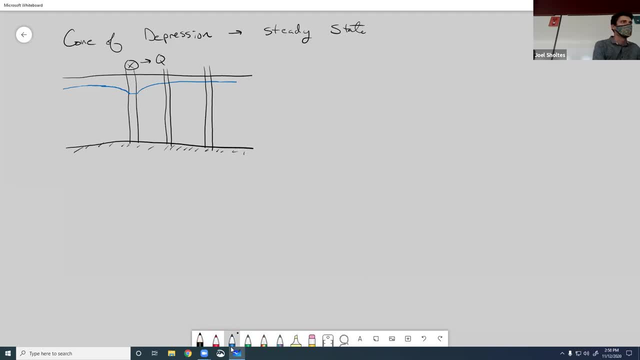 All right, we're going to define a bunch of things here. This would be the original water surface. is that dashed line? It's like: well, my roommate does the worst thing, Gross Like what, like from gas stations, or what I had to do- that was my first job- was environmental stuff. It was. there's some 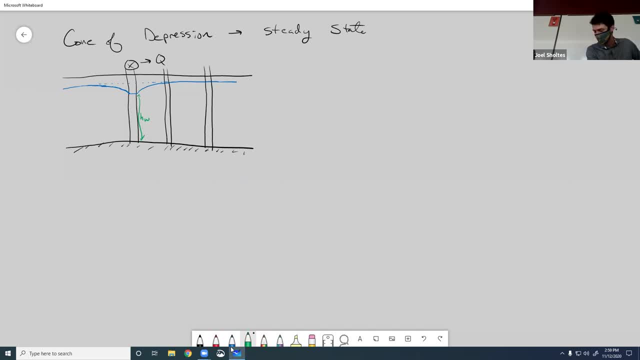 gross stuff out there: Diesel spill and just like it smells so nasty. Okay, and then we're going to define this as some distance are sorry, let me do this. The distances are going to be between the center line of the wells, Okay, so the center line of this. 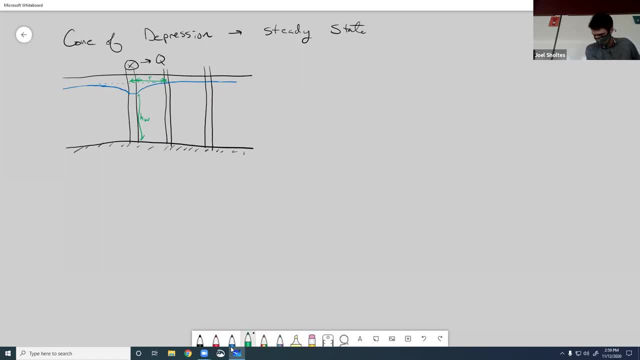 well And the center line of this well, The well diameter can actually make a make a difference, Or the well radius. So in this case this is the radius of the well And then we can have the water table height at some distance, some r distance away from the well. 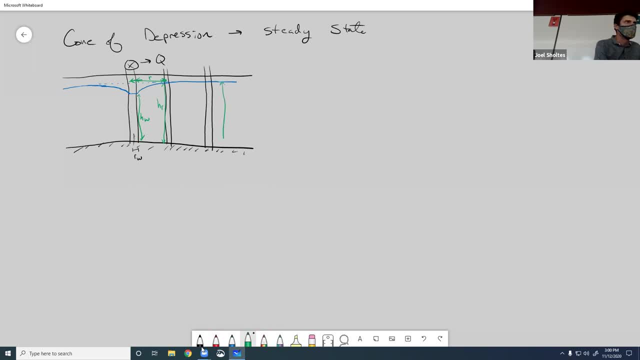 That's being pumped, And then we can have the original water table height or the initial water table height before pumping began, which is h? naught. And then we have the water surface slope, Which is d? h over d? r. So let's take a look inside the well itself. 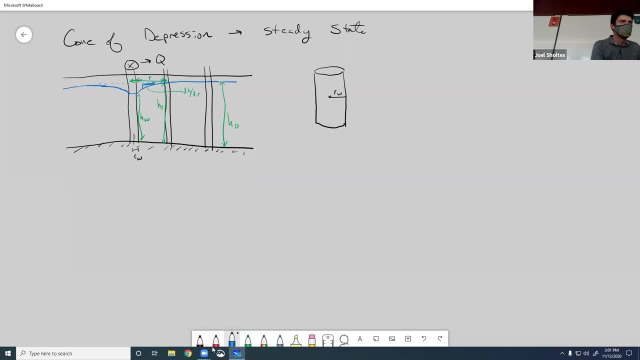 We have that radius of the well, We have the water depth in that well And we have the damper depth in that well, And we can define the area that the water is being pumped, And so the area is really just going to be this. 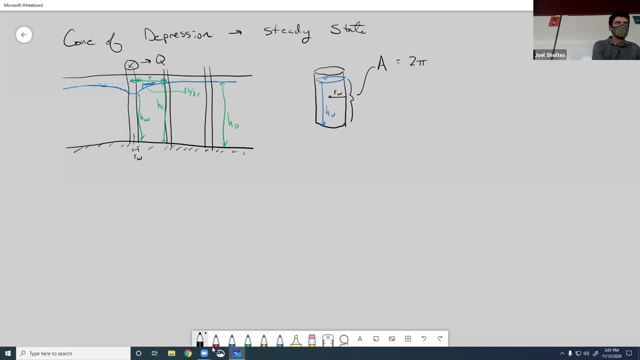 cylindrical area, right, The area that the water is being pumped out of, that well, so that's going to be the circumference times the depth, so just length times height. so that's the cross-sectional area that we're pumping water out of. and if we go back to Darcy's equation, we know that q is equal to negative k times, area times the. 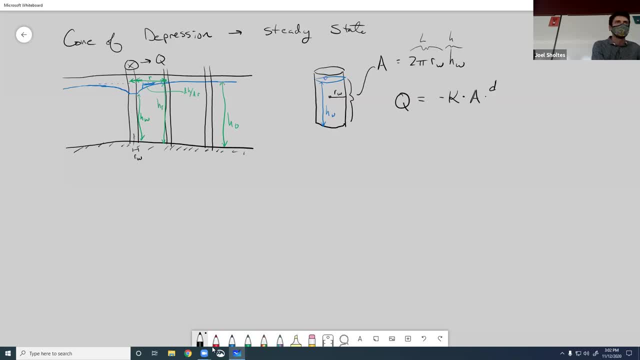 hydraulic gradient, in this case dh over dr, and so we can say that that's going to be equal to negative 2 pi rw, hw times k, times dh over dr. all right, and then ultimately, to solve this equation, we have to integrate it, because we want to get rid of this, this differential here, so that we can integrate the equation and solve for. 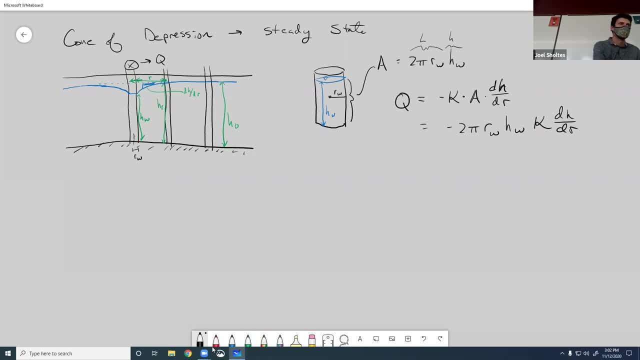 q and basically solve for this, this linear surface as well, based as a function of q. so if we know q and we know k, then we can calculate, if we integrate this equation, h as a function of r, vice versa. so we'll, we'll do some integration and then we'll end up with 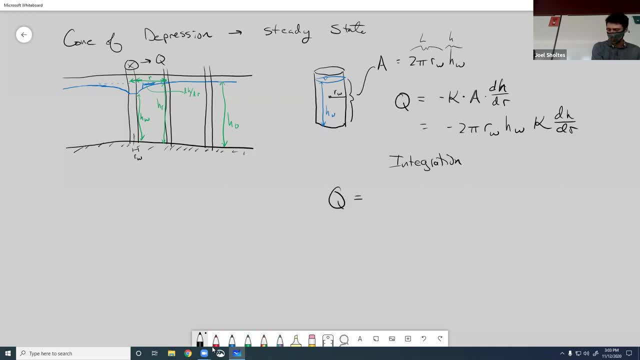 this cone of depression equation which says q is equal to pi times k, h minus hw, squared all over the natural log of r over r, dh over dr, and then we'll end up with this cone of depression equation which says q is equal to pi times k. 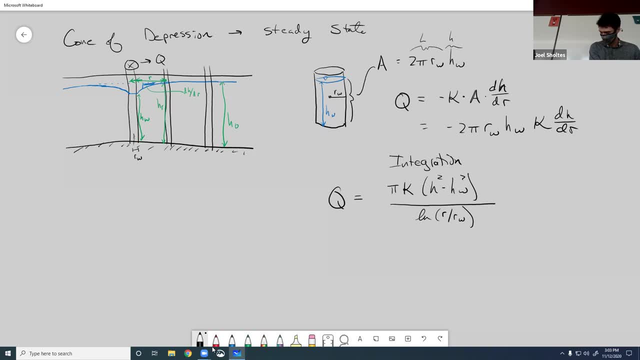 So integration gives us this: where we have HW is at the well and RW is at the well, and this is some distance R, right, and this is at R, And so you can define that water surface elevation H. ultimately, you're solving for H, right? if you wanted to find that water. 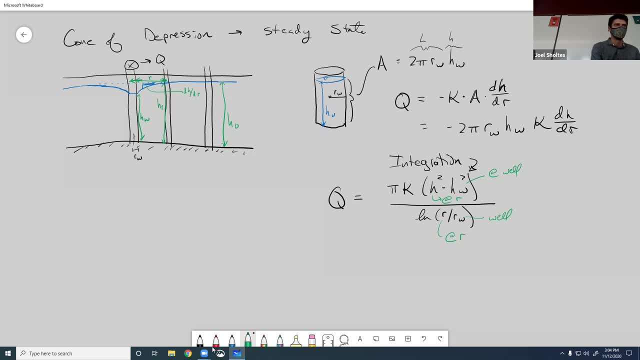 surface cone as a function of distance R and Q. Alternatively, you can say: given I'm pumping, say I'm pumping out 100 gallons per minute or something like that- right then I have my two observation. wells, I could tell you what the H is going to be in this well, and 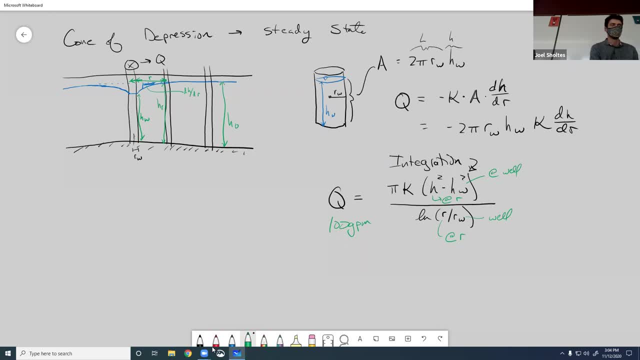 what the H is going to be somewhere else, at some radial distance away. So this is when you have an observation at the well and then some distance away from the well, or you could base this off of just two different observational wells and that's. 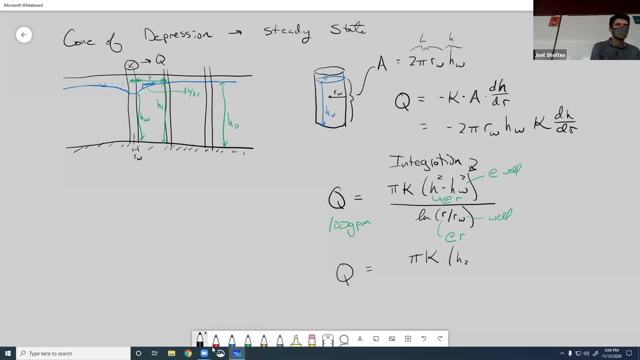 just going to be a very similar equation, which is pi K, H2 squared minus H1 squared all over LN of R2 over R1.. In which case, this could be well two, and this would be well one. It's defined, you know. what you measure is the. 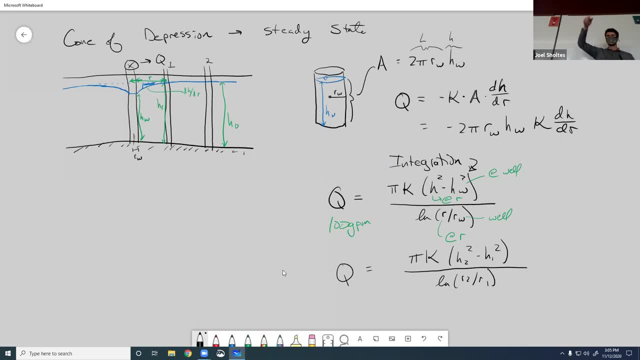 depth from the well casing top right. So you put a little tape down there and then it hits the water and it beeps, and then you read off the depth to the well So you can get, you can set H as some arbitrary data and you can say: okay, my aquifer is. 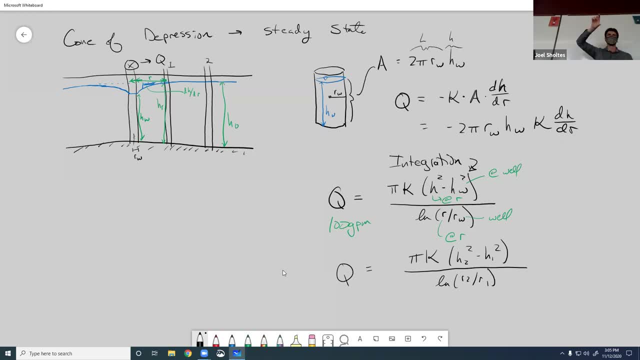 going to be 100 meters deep, and then you just subtract what you measured from that. So it's all in terms of H. You could rewrite that in terms of depth to the well, but we put it as H. How do they determine that? 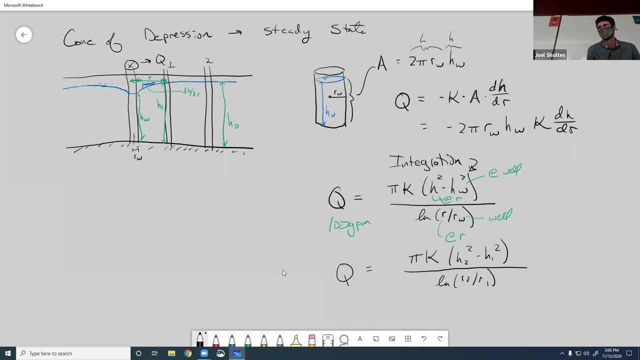 Yeah, well, log in a really deep, well, you know, and you're like: okay, clay, clay, clay, sand, sand, sand, gravel, gravel, gravel, sand, sand, sand, clay, clay, clay, and you're 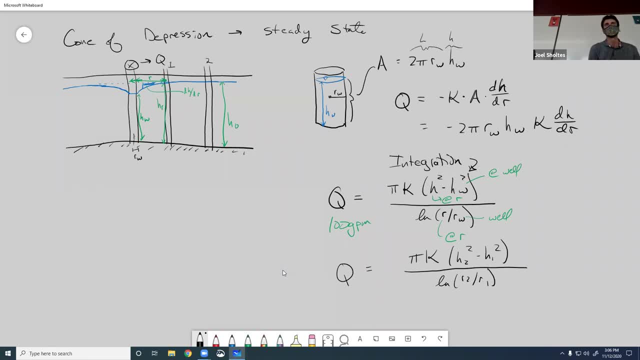 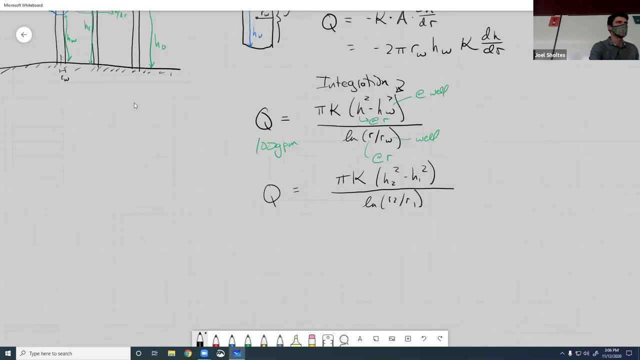 like, okay, that's my bottom. Yeah, that would. that would be the way to do it. All right, let's look at a confined aquifer. It's going to be a very similar, just a little bit different, And we'll draw our confined aquifer. 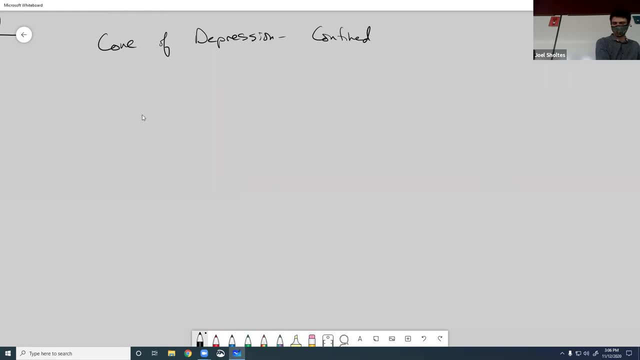 I'm going to draw kind of a big, big picture: confined aquifer. So we'll have the ground. we'll kind of start up in the mountains and we'll come down to the plain. So this will be our ground surface. We'll have some sort of aquitard. 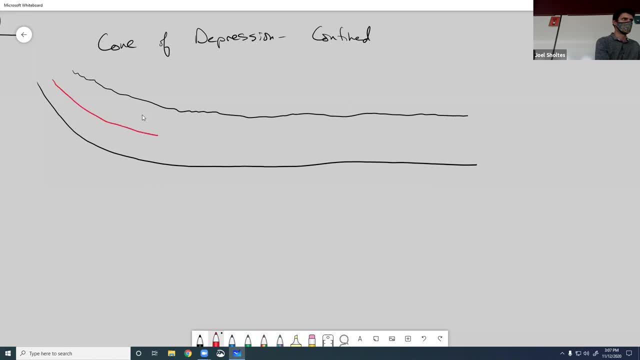 I'm going to make it red. So that's our aquitard, And then this would be another aquitard at the bottom of that. So here's our aquifer, our confined aquifer, And somewhere up here we have a water table that has a free surface. 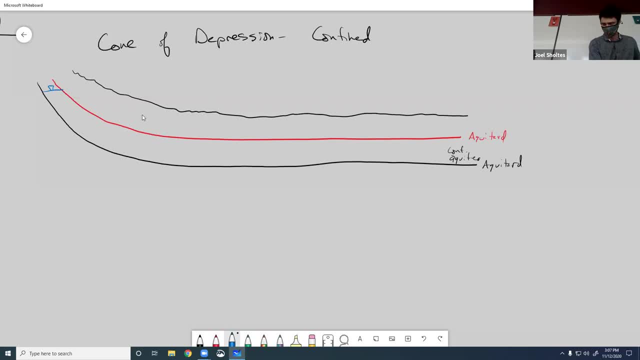 But as we go down here it starts to be pressurized, right, We get those artesian conditions. So there's a potentiometric surface that you know essentially. let's say, I'll just kind of draw it like this: 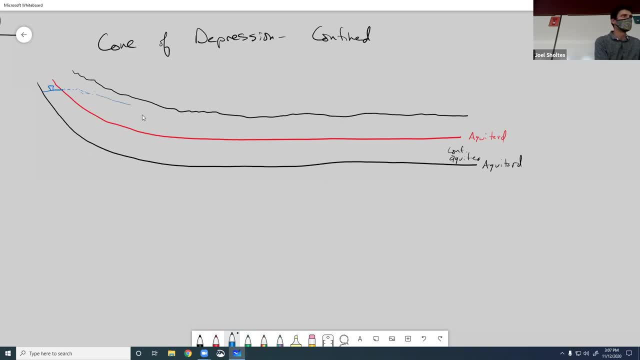 Um, what What? Um okay, um, um, um, um, um, um, um. just a sec, Say that again. So this would be um you always for confined aquifer. you always need to have a sandwich. 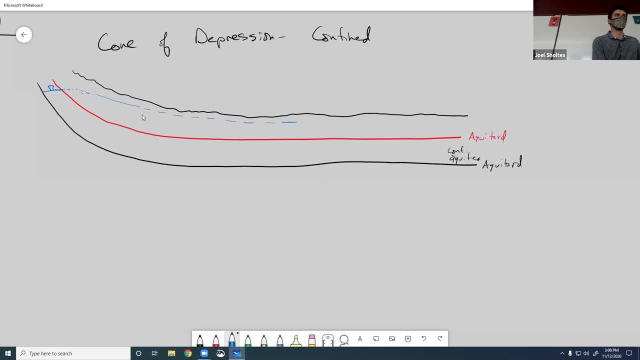 So you have one aquitard and another. so this, this sandwich, is where the confined aquifers in, This is where the pressure builds up This kind of acts, like your pipe walls. So the aquifer is here and the water is moving down this way. 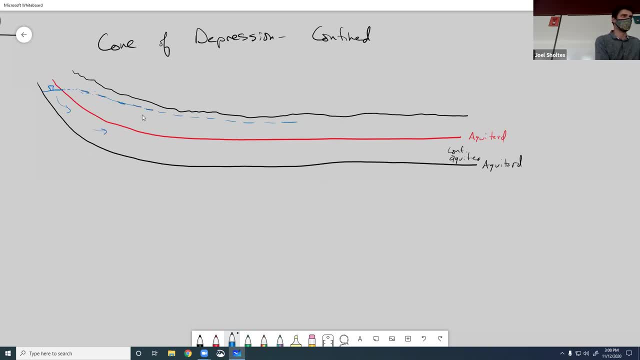 And you've got that potentiometric surface, which is basically the, the pressure that exists, and if you were to put an observation well in here, the water would rise up to this potentiometric surface. So if we put some wells in here- I'm just going to do two wells- 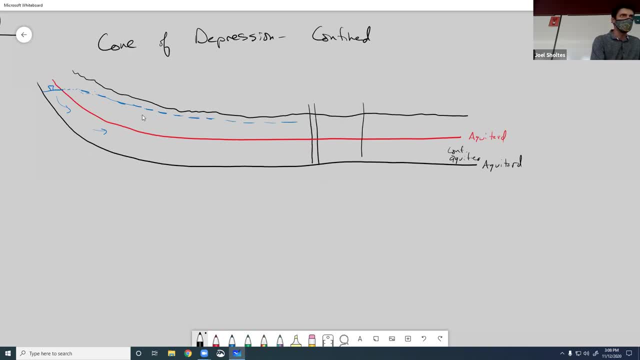 this time and we start pumping. Instead of a cone of depression from the water table, we get depression in the potentiometric surface which manifests as the free surface in a well. So it's really just like an imaginary cone of depression. So wherever you put that well in. 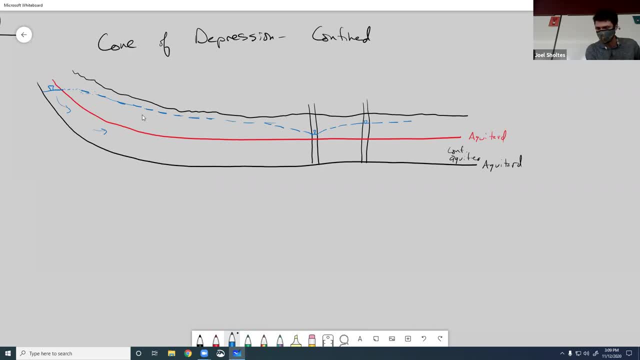 the water is only going to rise so far based on that cone of depression And if we're pumping out at a certain flow rate out of that, well, we can do. let me just define this as potentiometric surface And we'll do some similar calculations here. 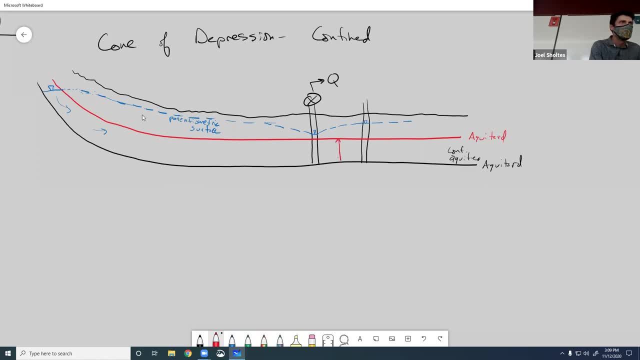 but we'll introduce a new parameter. In this case, we have the thickness of this aquifer, the confined aquifer, which is b. We'll have the height of the water in the well. We'll have the height of the water somewhere else. 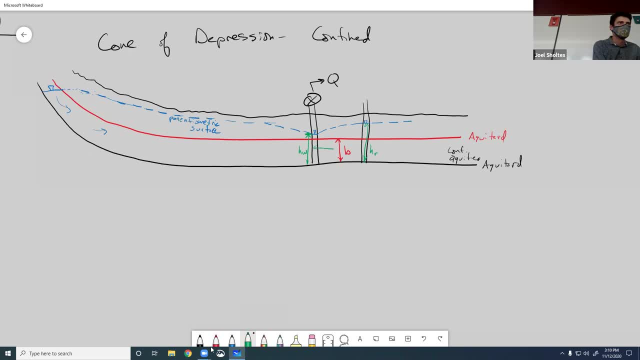 We'll just call that h sub r And then we'll have a radius between the two well center lines. So we're going to do: for each point that we get above and below in the new equation, we'll get h minus hw, So that'll be h minus hw over the first equation. 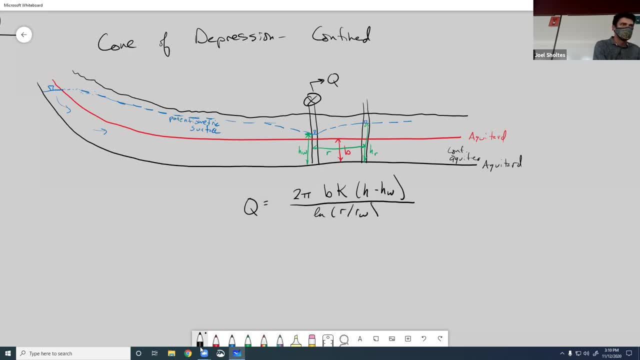 And then in this case, our cone of depression. equation Q is equal to two pi B times K, h minus hw. So they're not squared this time ln of r over rw. So we'll just look at this. We'll take an odd area to its lowest point. I'm just gonna try and write this down as well. This is the most beautiful equation. Frieden's equation will just keep spinning on this. I'm going to take a really long time here to test it a few times, just to make sure that my answer is accurate. 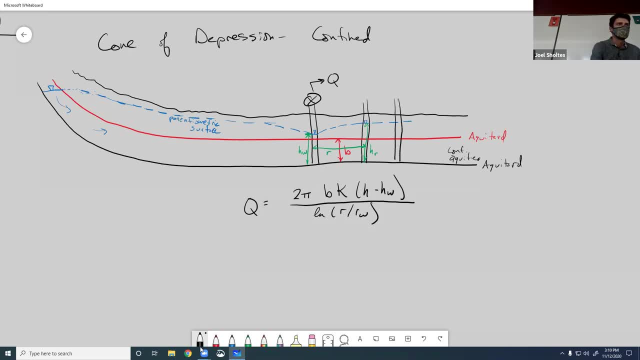 And I'm going to take a little bit of time to calculate the value of information I'll get. The most important thing is that we're going to give some of this data to all of our colleagues. Alternatively, if we had two wells, this would be: Q is equal to 2 pi, E, k, H2 minus H1. all over ln. R2 over R1.. 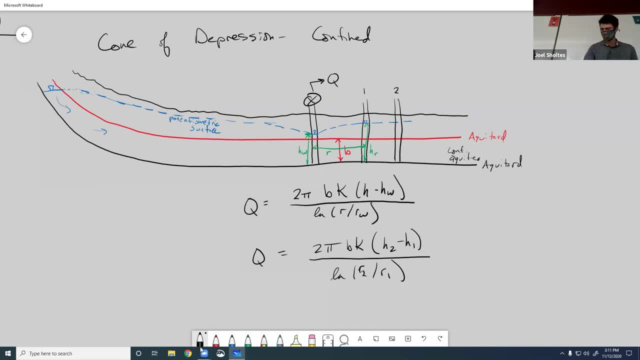 All right. so this is the kind of classic Effie groundwater kind of question. so that's why we're doing it and it gives you kind of a basic idea of steady-state flow. The way this would work is: we set up a well, you start pumping and you're pumping at a constant flow rate. 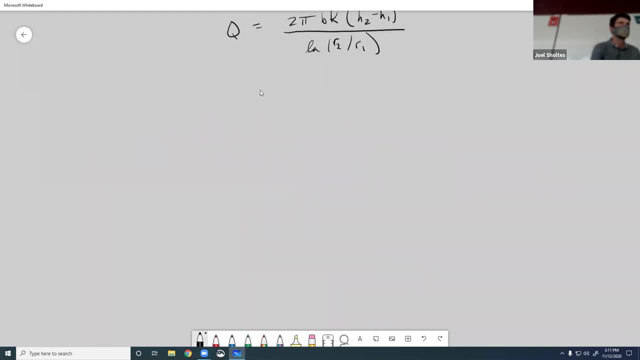 And so there's two questions we could ask or two kinds of problems we could solve. So the first problem would: be given that pump rate Q, which is steady, let's calculate the drop in well elevation or groundwater elevation. Okay, 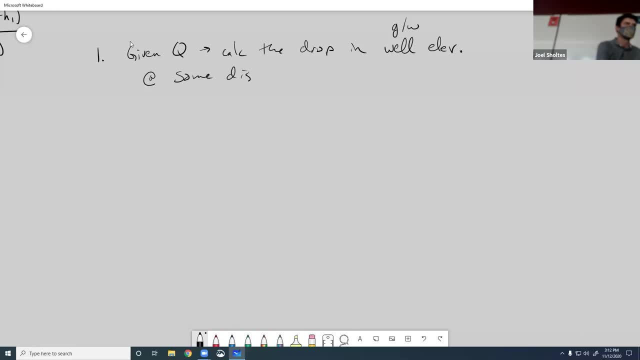 So let's say I'm pumping at some distance, So this is like a drawdown. you know how much am I going to impact my neighbor's well, Or am I going to create a reverse gradient so that all of a sudden water is starting to flow from a certain area, that where it didn't before? 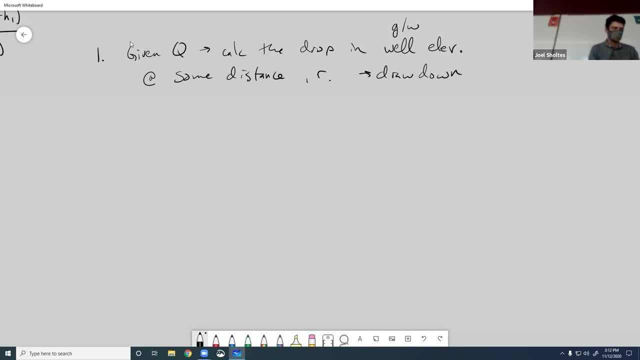 Because you can kind of reverse directions of groundwater flow. We talked about that example on Tuesday where you could potentially be drawing water from a certain area. but you can't do that. You could potentially be drawing water from a surface source that you didn't want to go into your well. 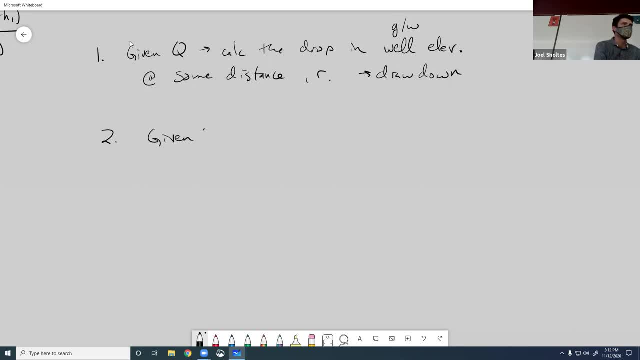 The other thing we could do is we could say, given Q, H1,, H2, what is K? So we can actually calculate the hydraulic conductivity based on this steady-state. And so steady-state is where we turn the well on. we pump at a constant flow rate for days, right. 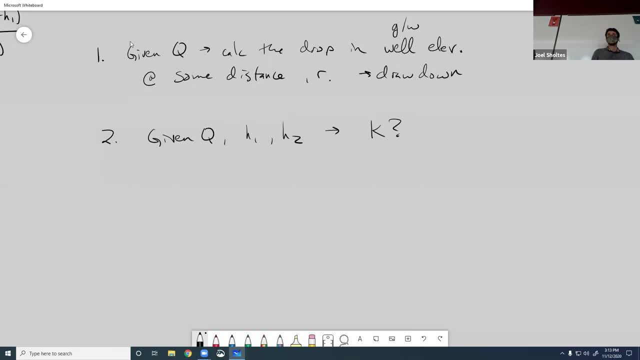 So it's going to take days, weeks, depending on the hydraulic conductivity of the aquifer. If it's a really low hydraulic conductivity, it might take days, weeks, months to reach a steady state where that groundwater is not drawing down slowly over time, increasing the slope. 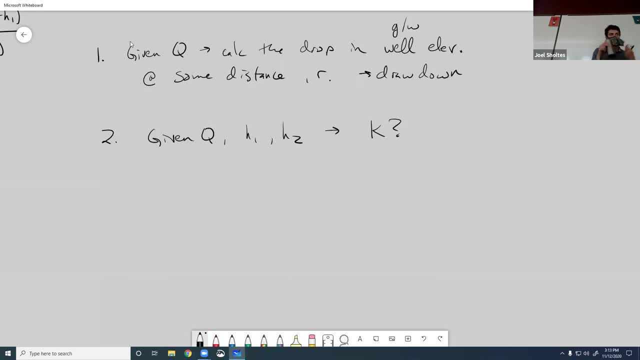 If it's a really low hydraulic conductivity, like sand and gravel, it might take days. However, sometimes we don't have days to pump and test things, So we can use unsteady equations and unsteady relationships to measure properties of the aquifer based on hours-long tests or day-long tests or something like that. 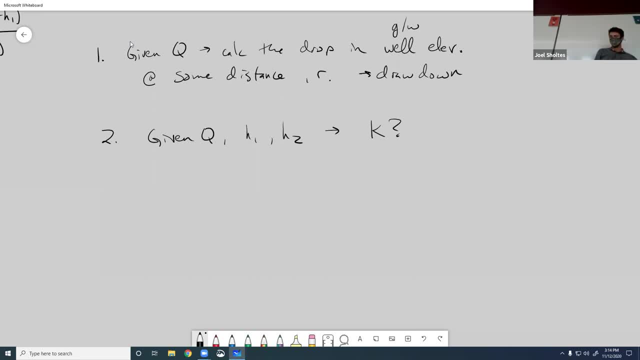 And that's called pump testing and slug testing. We'll talk about that in class on Tuesday And I'll also do an example, because we ran out of time. So I'll do an example on Tuesday of this And then we'll talk about something else. 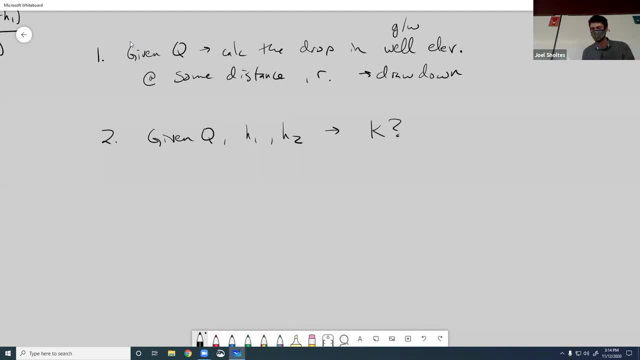 Slug testing and pump testing, Basically aquifer testing. All right, So I will be available for office hours on Zoom tomorrow from 1030 to 1130.. If you need to talk to me outside of this time, just email me. 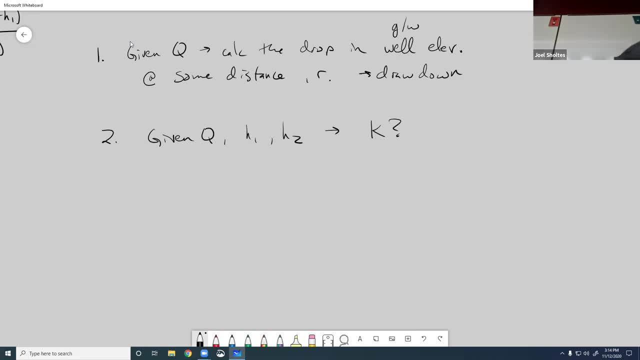 We can set something up. I'll give you your exams back And at GardenValve I can scan yours and send it to you, If that works. Yeah, that's fine. Thanks, Don, I can also hang around if you guys have any questions here. 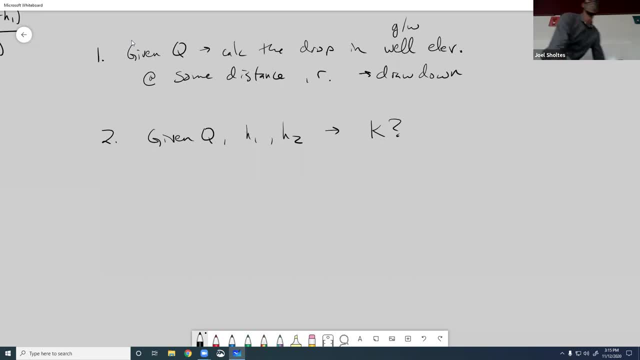 And Val and Edgar. I'll scan yours and send it to you in the next few minutes. See you guys on Zoom. 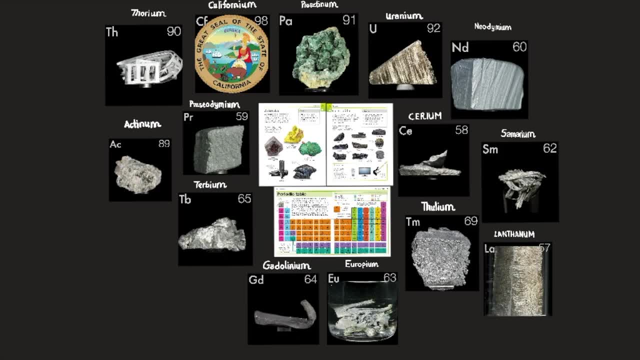 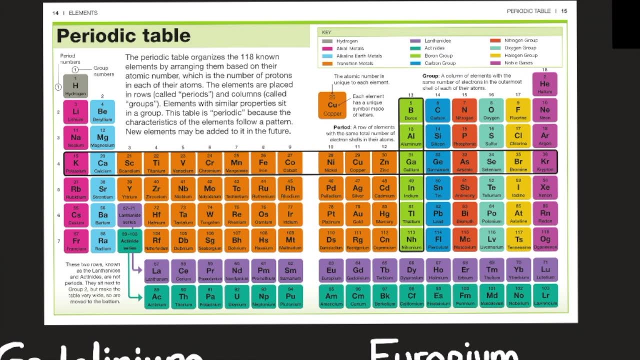 Hello everyone. today we're going to talk about the actinides and lanthanides on the periodic table. So here we have the periodic table. Here's a brief review. The periodic table organizes the 118 known elements by arranging them based on their atomic number. 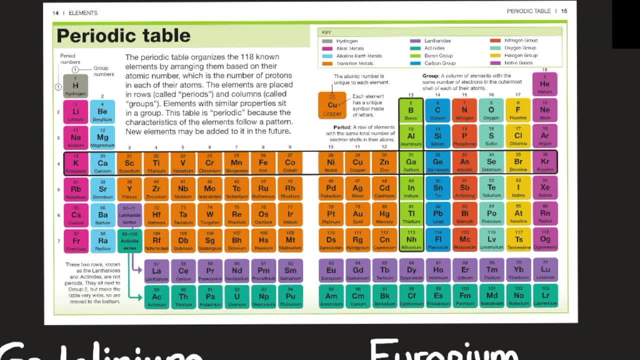 which is the number of protons in each of their atoms. The elements are placed in rows called periods, and columns called groups. Elements with similar properties sit in a group. This table is periodic because the characteristics of the elements follow a pattern. 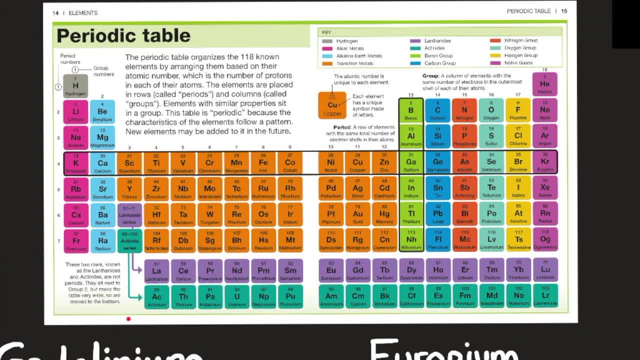 New elements may be added to it in the future. So these two rows known as the lanthanides and actinides are not periods. They sit next to group 2, but they make the table very wide so they are moved to the bottom. 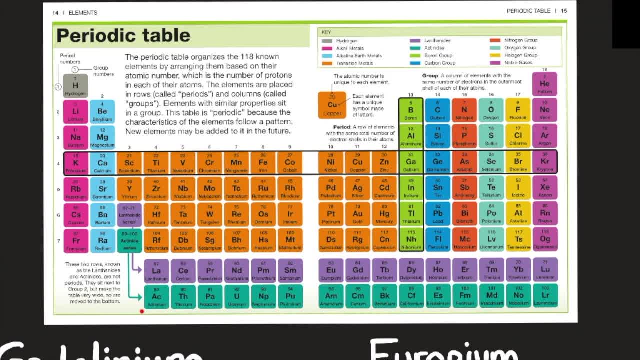 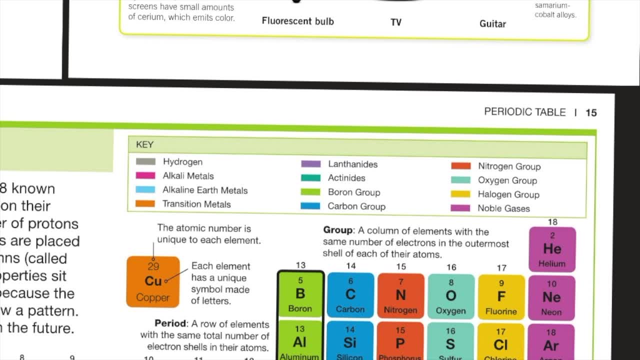 So here are the lanthanides and actinides. Here's lanthanum and actinum, which is why they're named lanthanides and actinides and are the ones in front of the whole region right here. So here we have the key hydrogen alkali metals, alkali earth metals, transition metals.